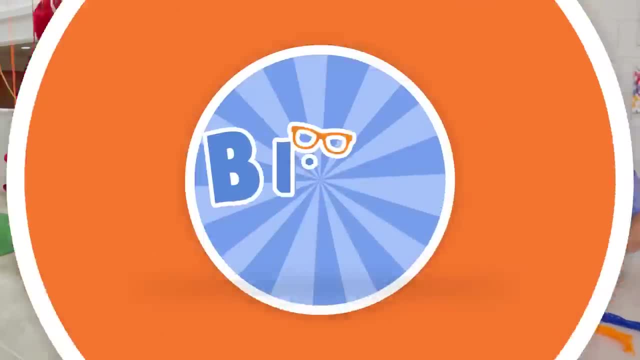 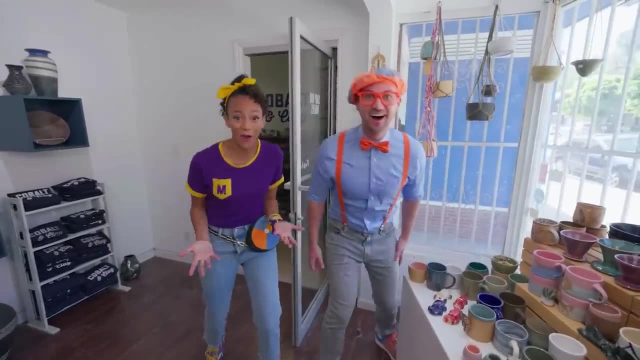 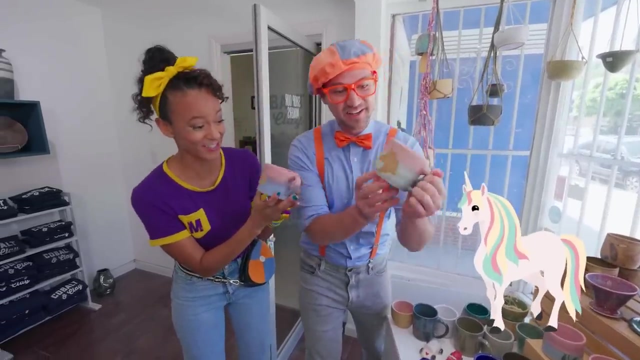 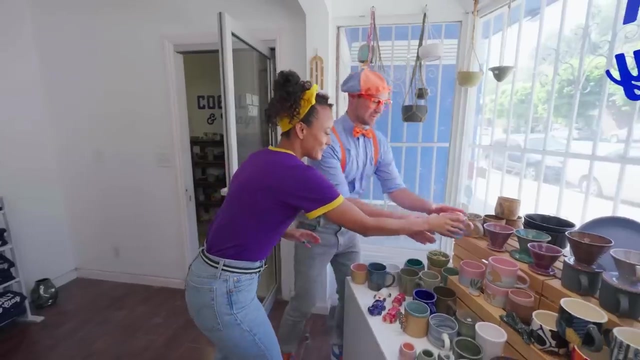 So much to learn about. It'll make you want to shout: Flippy. Wow, Oh, Mika, cool. Yeah, this room is filled with different art pieces. Yeah, check it out Here. do you want one? Oh, yeah, thank you. Wow, unicorn mugs, These are so cool. Cheers, Yum, Whoa, there we go. Nice and gentle- Yeah, there we go. Whoa, check it out Cool. 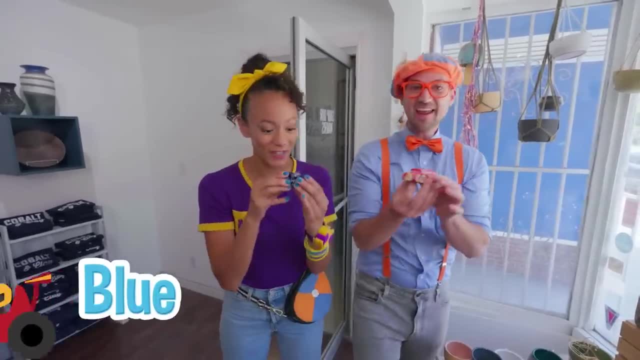 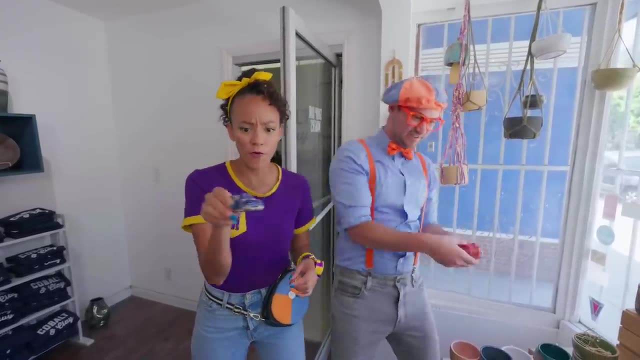 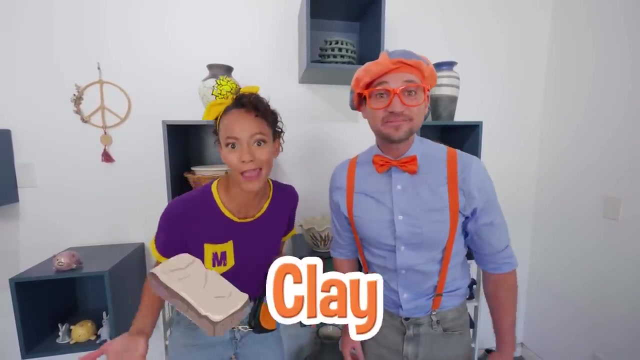 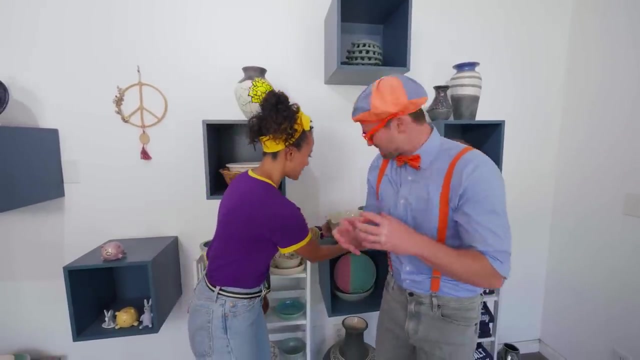 Cars- Mine is blue, Yeah, mine is red- So cool that you can even make cars out of clay- Yeah, awesome. Well, this pottery is so cool. New pottery is an art piece that's made out of baked clay, Yeah, or other types of stoneware. Yeah, it's really cool because it starts soft and squishy and then it ends up like this: It's nice and hard. Yeah, Oh cool. Hey, look at this. Whoa. 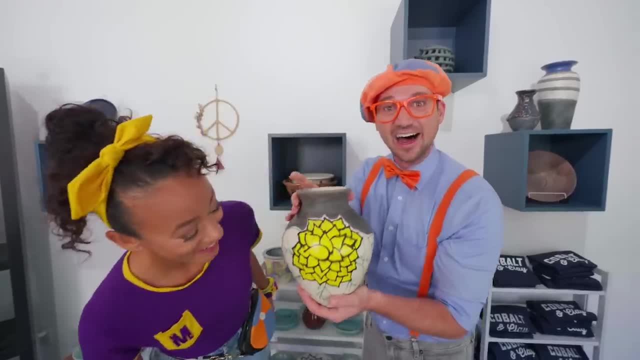 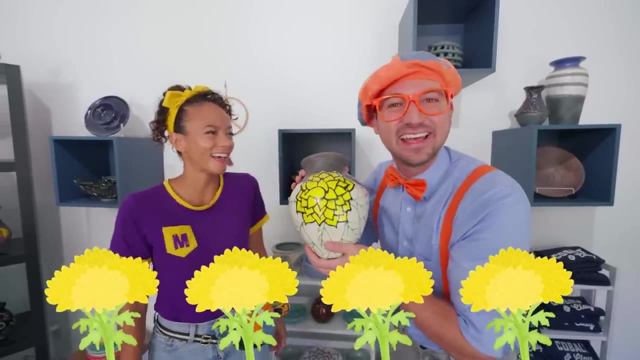 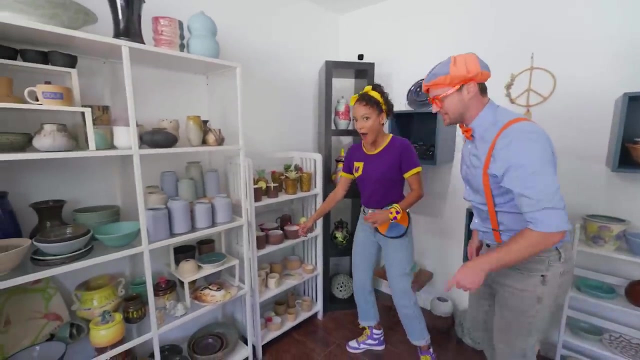 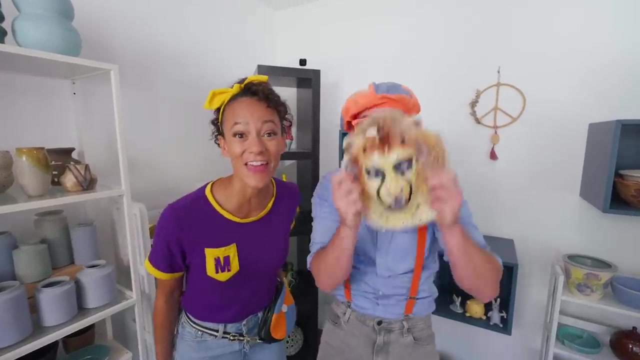 Oh, I'm being very careful when I hold these. Good job, Yeah, A yellow flower. Yeah, it's so pretty. Yeah, Smells just like clay. You're so silly, Whoa cool. Whoa, Do you see what I see? Yeah, I do. Whoa Ready, Do you know what animal that is? A lion? Yeah, Will you act like lions with us? Yeah, 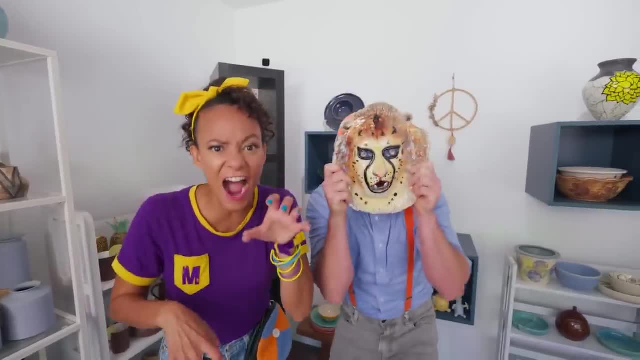 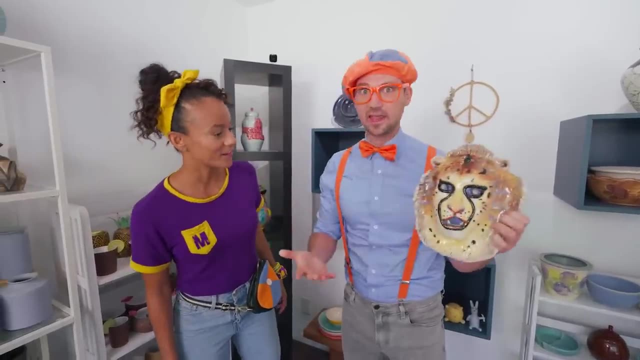 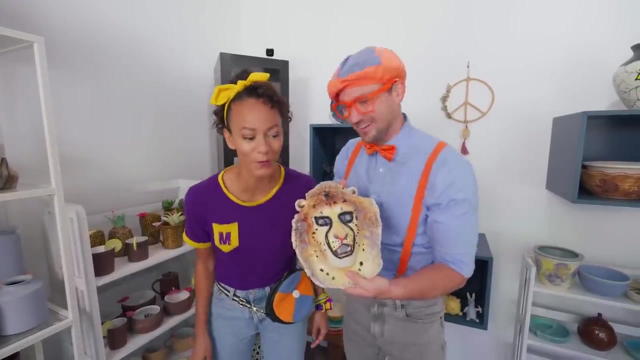 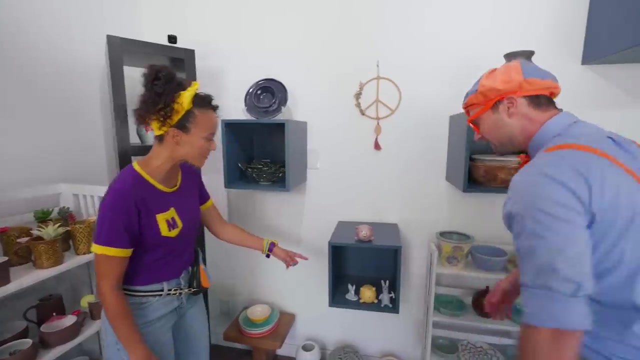 Whoa, So cool that an artist made this lion out of clay. Yeah, it's pretty awesome. Yeah, and it's so colorful too, They must have painted it. Yeah, look at the blue eyes. Whoa, Kale, very gentle when I set that down, Nicely done, Oh thanks, Hey, Blippi, there's more animals down here. Oh, yeah, you're right, Look a bunny rabbit. 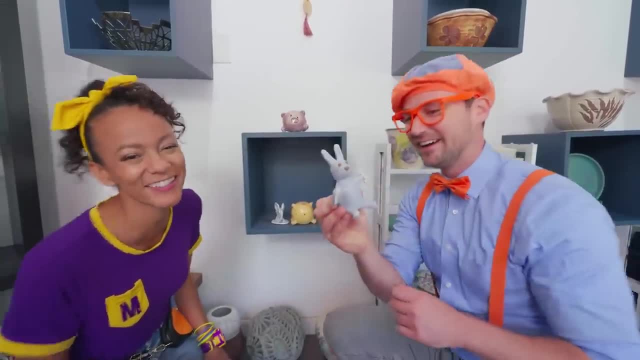 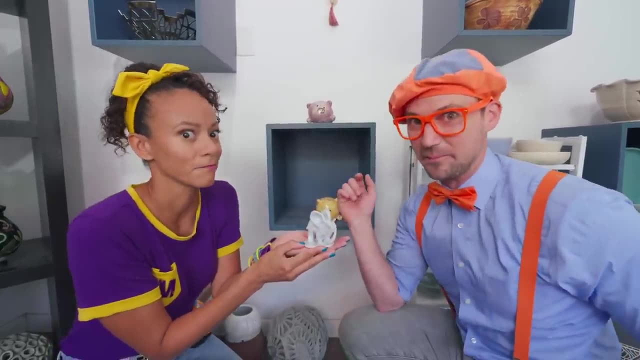 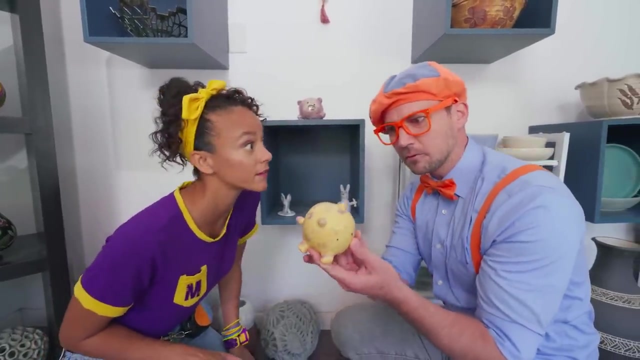 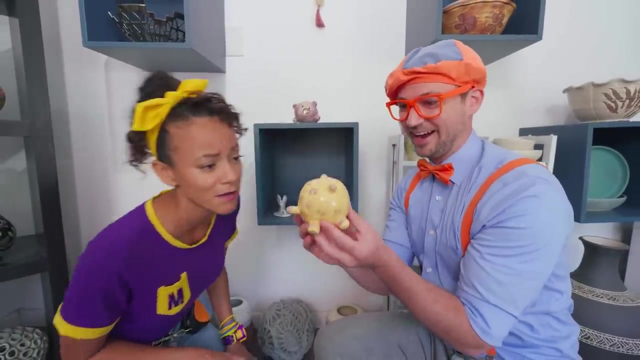 Aw, Nice little carrot right there, It's so cute. Oh, what about this little elephant? Aw, Little elephant but big ears. You got that right. Oh, and look at this one. Oh, what is that, do you think? Huh, maybe a leopard. Oh yeah, and it's really big, almost like a blowfish, but it's not a fish. Yeah, so artistic. Yeah, really cool. You can make anything you want. Yeah, and it's so cool. 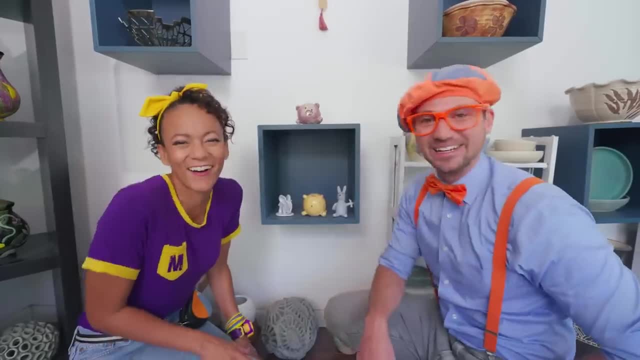 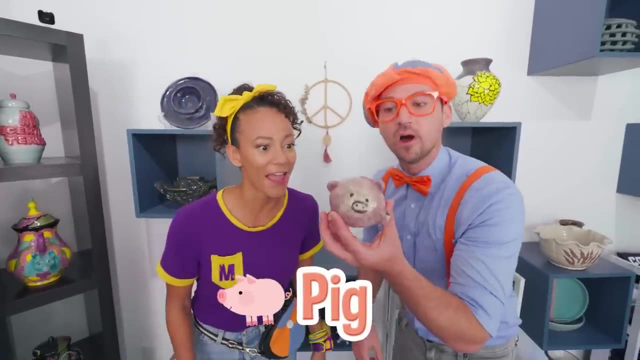 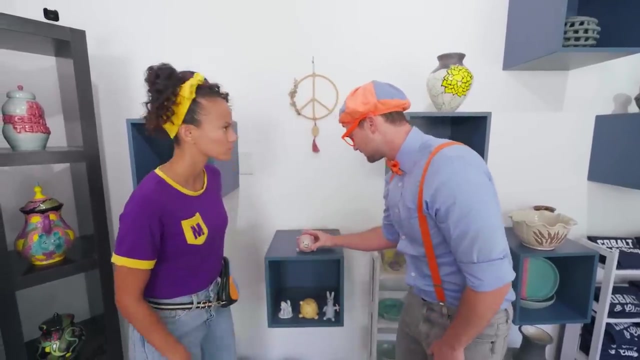 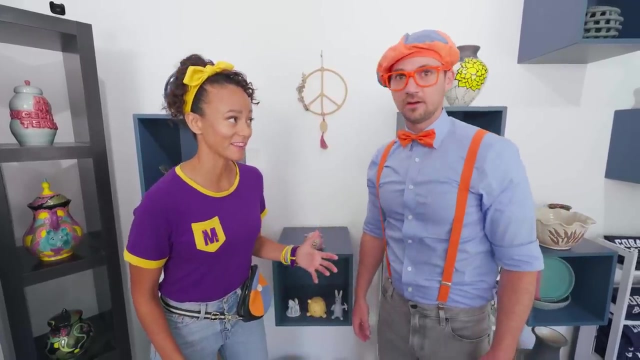 It's so cool that these animals, Yeah, are nice friends together. Aw, so cute. Yeah, Oh, look, there's another one up here. Oh, interesting, Looks like a pig right, Yeah, and purple, one of my favorite colors, Oh yeah, Oh, but wait a second, It's all alone, Yeah, and it looks like there's some space for other animals. Are you thinking what I'm thinking? Yeah, Lunchtime- No, Oh. 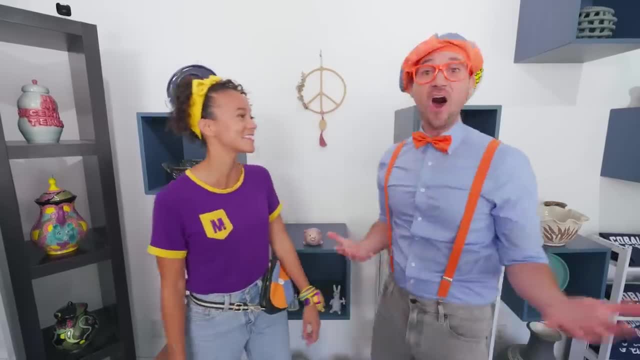 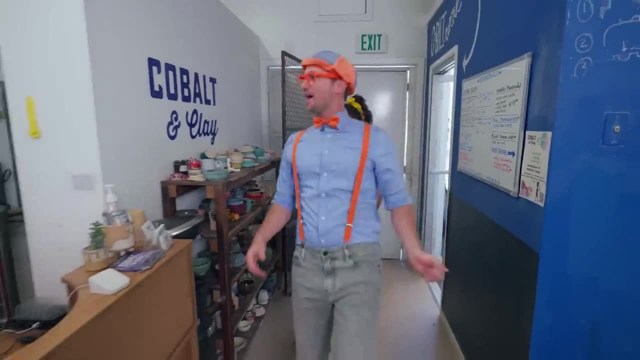 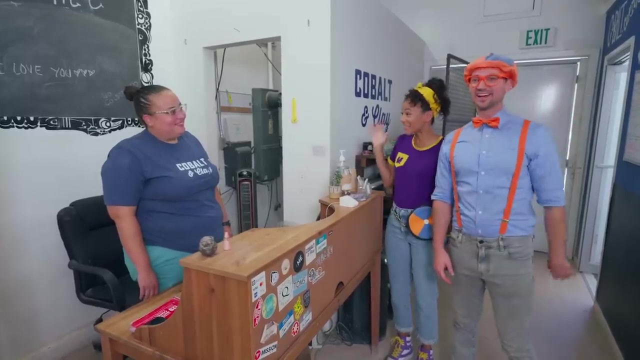 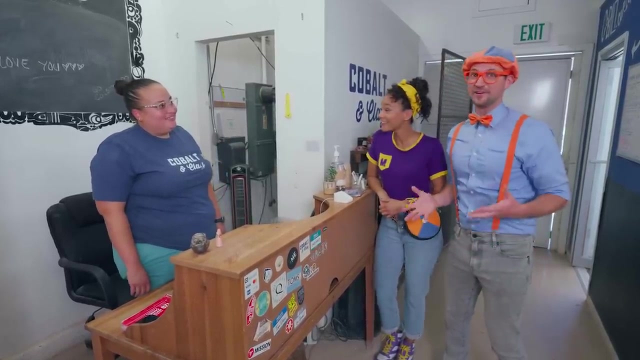 We can make this pig some animal friends. Oh, that's a great idea, Mika. Yeah, let's do it. Yeah, Oh, Oh, Oh, hey, who are you, Hi guys, Welcome to Cobalt and Clay. My name's Nicole, Oh, nice to meet you. I'm Blippi Hi, and I'm Mika, Oh, So what do you do here? I'm the owner and instructor, Oh, cool. Well, you might be the perfect person to ask: Do you think we could make some pottery today? Of course, Oh Yeah. 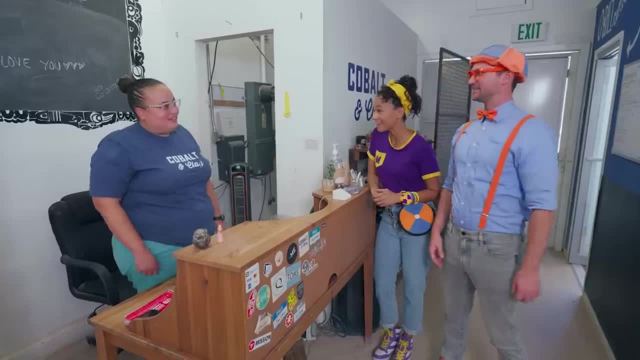 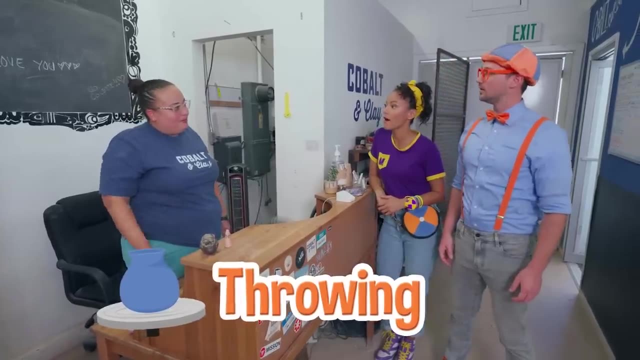 I want to make some animal creatures Awesome. Well, would you like to hand build or throw? Hmm, What's the difference? Well, hand building is where you use your hands to sculpt and throwing is where we use the pottery wheel that spins. Oh, Oh, Could we do both, Of course. 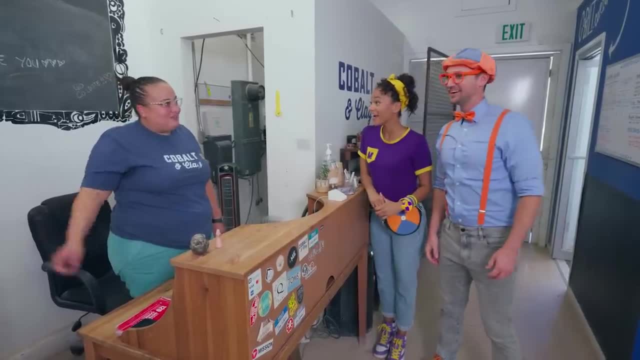 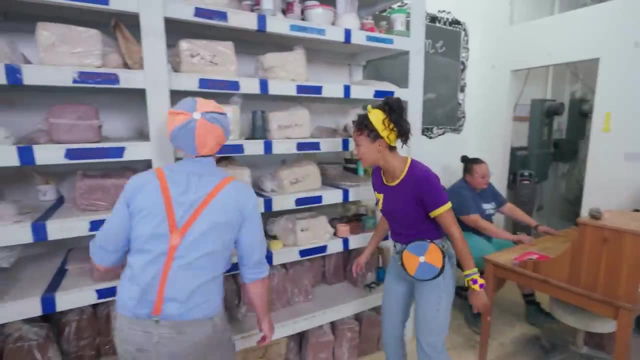 Yeah, Yeah, How do we get started? You guys want to grab some clay and I'll meet you at the wheels. All right, Okay, Thanks, See you later. See you, Oh cool, Oh, look at all this clay: Blippi, Wow, Big blocks of clay it looks like. Yeah, Oh, look at this. 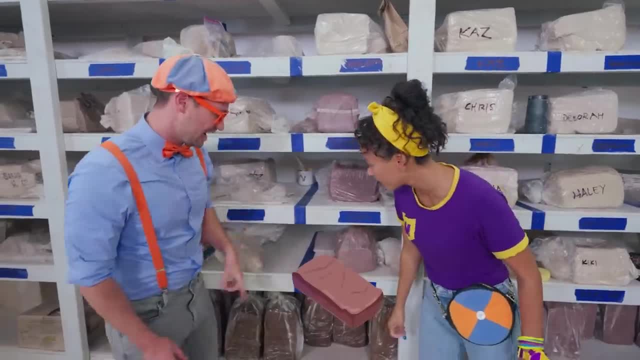 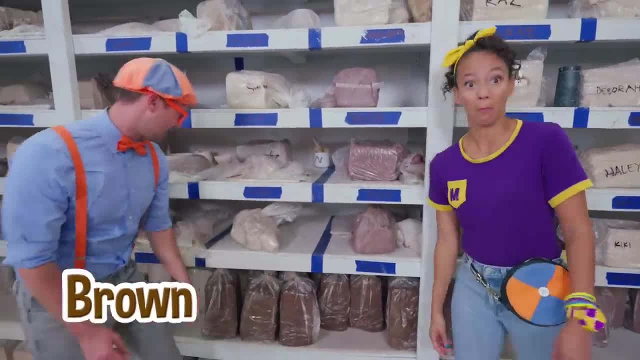 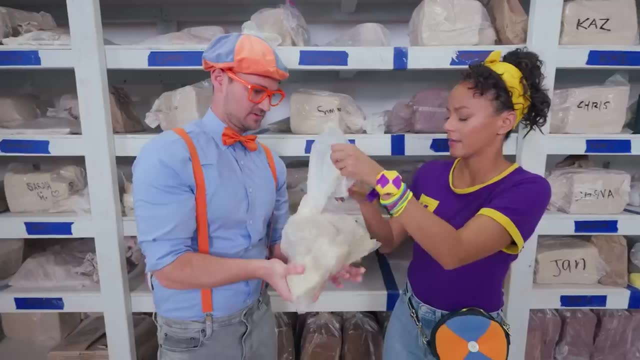 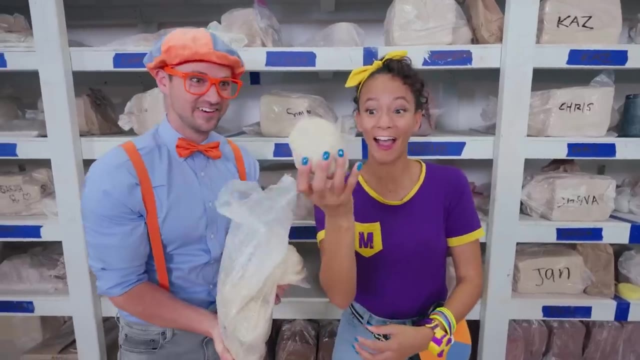 down here. Oh, this was like a dark brown, Oh, yeah, Oh. and look at these. Oh, A nice tan color, Yeah, and the shape of balls it looks like. Yeah, interesting. Let's look inside. I wonder if they're the perfect size. Oh, check it out. Oh cool, Yeah, There you. 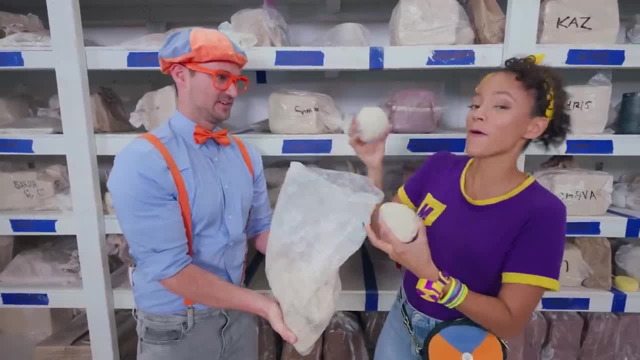 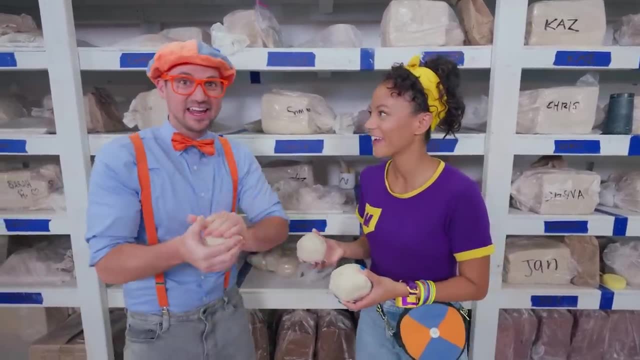 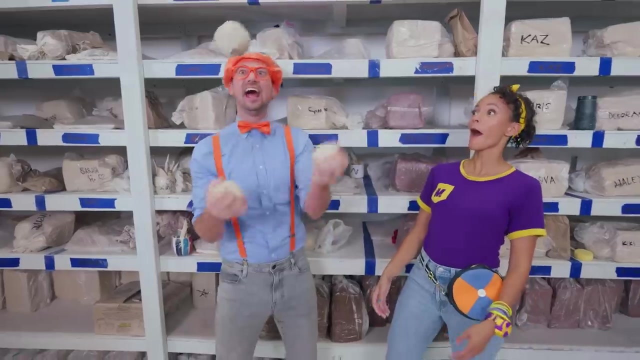 go. One for you, Oh, thank you. And one for me, Oh, cool. Oh, and I have a great idea: Whoa. And since they're pieces of clay and they won't get ruined if they fall on the ground, I know what you're going to do. Yeah, Here we go. Go, Blippi, Whoa. Nice job, Thank. 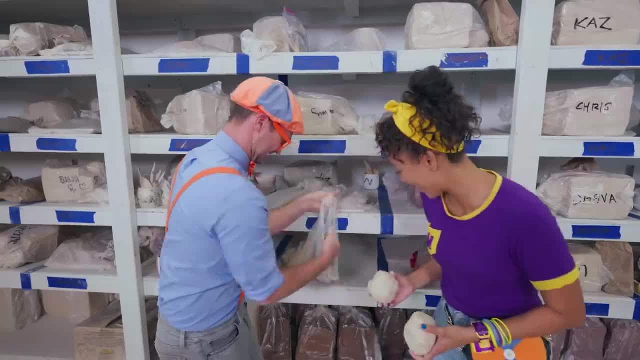 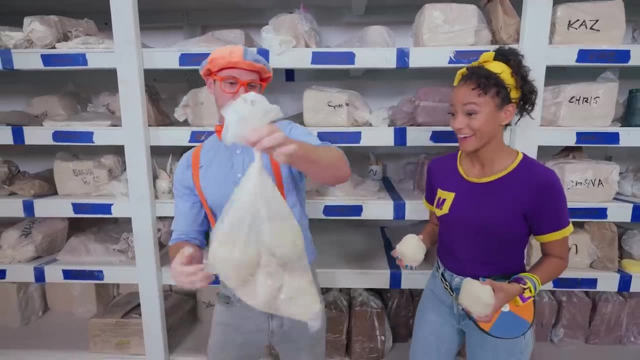 you very much. I should probably put this third one away. right, Yeah, Let's seal up the bag, so then you don't dry out. right, Good idea. All right, Nice twist. All right, There you are. There we go. All right, Check it out. 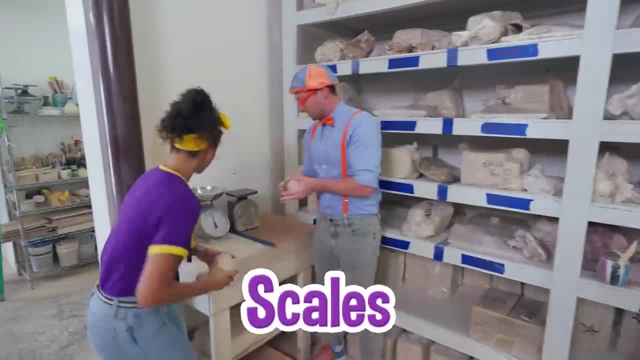 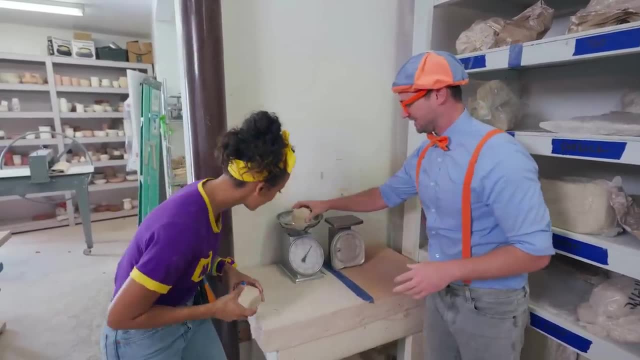 Oh, scales, Yeah, Whoa, We can weigh our clay. Yeah, Do you want to go first? or me? Oh, you go ahead. Oh, thanks, Mika, All right, Hey, there we go. Oh yeah, Looks like one. 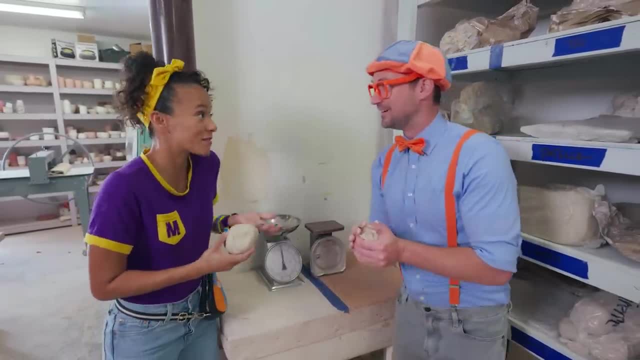 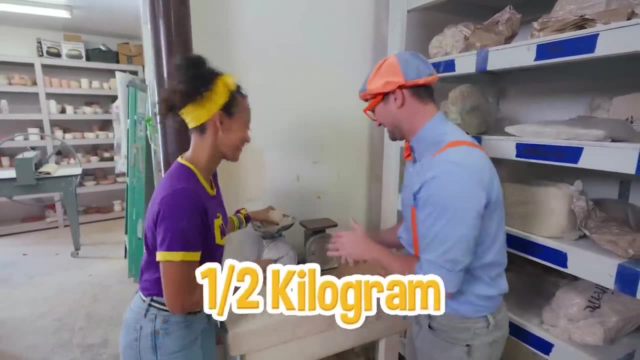 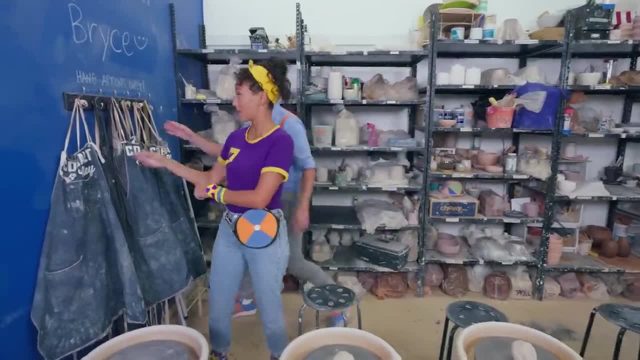 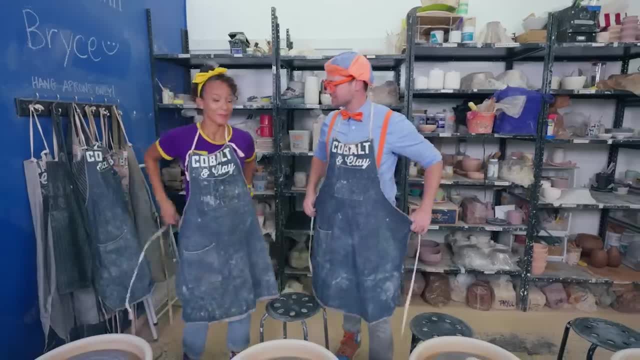 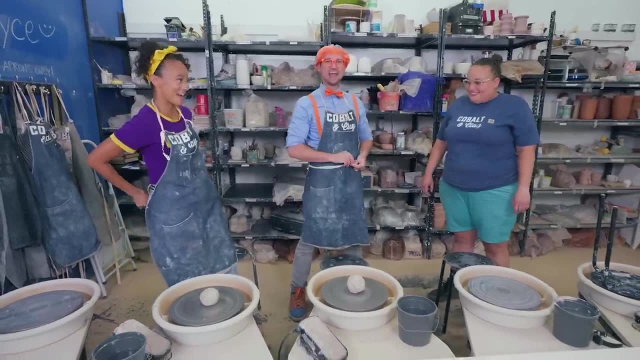 this will protect our clothes. Yeah, and it even says cobalt and clay. Oh, cool Matching aprons. Yeah, Oh, hey, Hi guys. Hey, Nicole, Are you ready to throw? Yeah, Throw clay. So I'm going to go over a few things that we're going to be using. So we have a bucket. 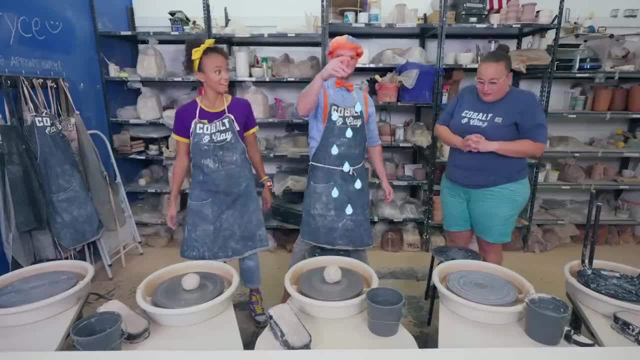 of water here. that's going to help the clay glide through our hands, Uh-huh. And then the way the well works. there's a foot pedal on your table. You're going to set it on a set it on the floor and that's going to control the wheel speed. okay, do we sit down? yeah, you're. 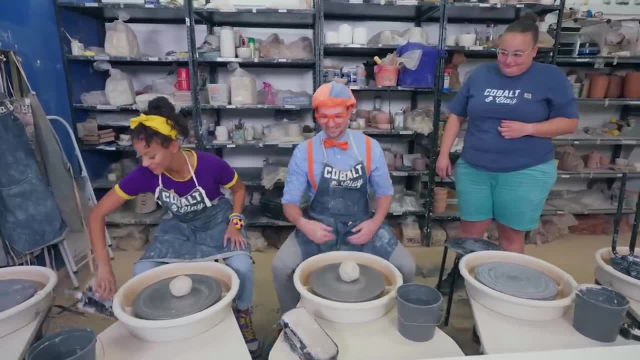 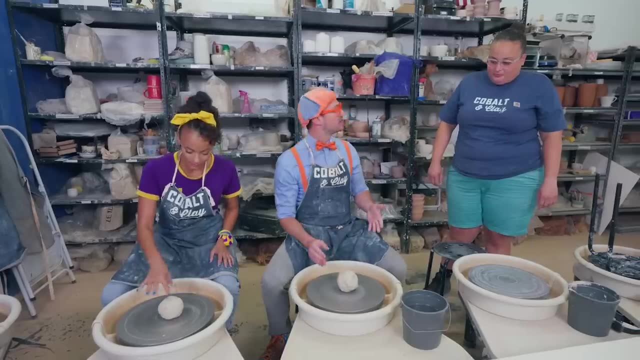 going to sit on your stool- okay, nice and relaxing. oh okay, pebbles on the floor and that's what you use to control the spin. and then what about the clay? so you're going to take it, you're going to smack it in that center circle, you'll tap the sides really well, seal the base, and then you'll 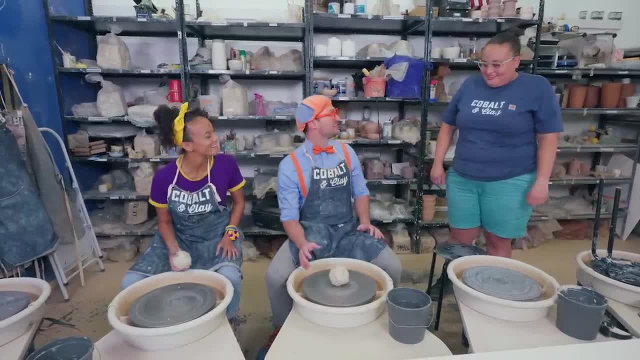 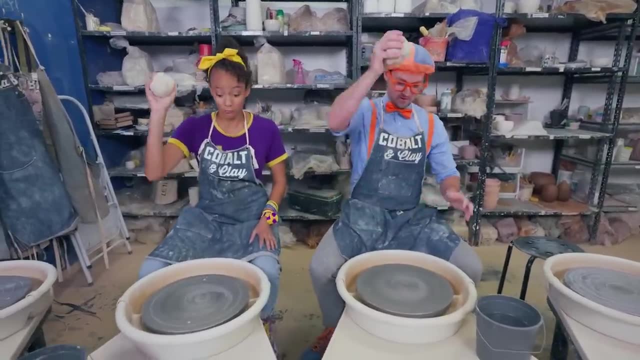 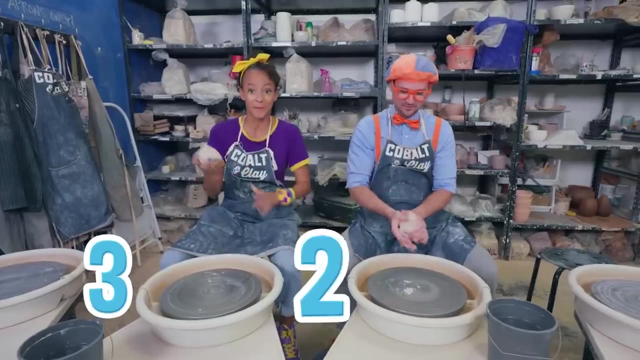 just start to mold. your piece sounds like fun. thank you so much. okay, i'm going to set up our next station. all right, thank you see. ya, okay, ready to throw it? ready to throw? whoa, i missed the center, me too. we should probably do that again. oh, whoa, three, two, one, yeah. 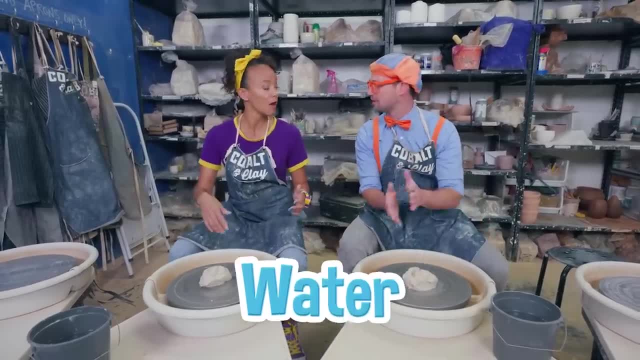 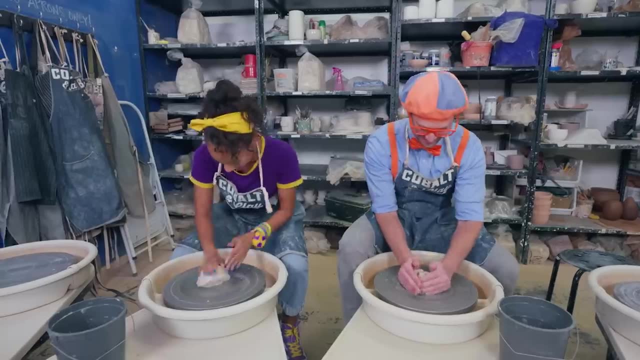 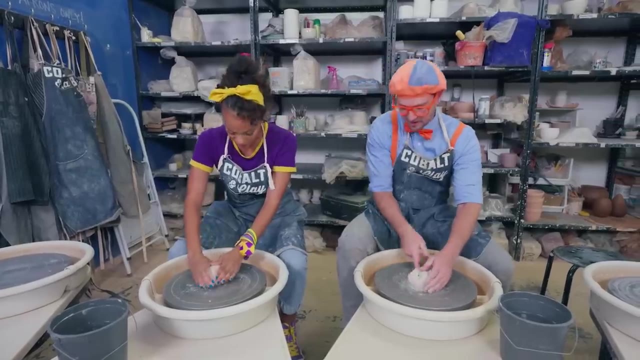 nice, okay. and then i think she said to use some water on our hands, right, what are our hands? okay, water, our chance, water, our hands, water, water, water, water. okay, there we go. all right, smack it, oh. and then she said: seal it, right, oh, so maybe push it down. i think we go around the edges like this: 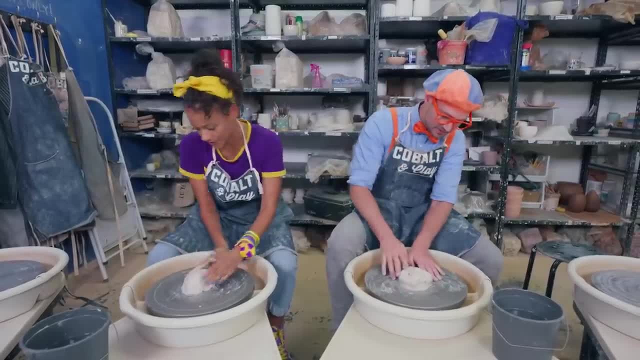 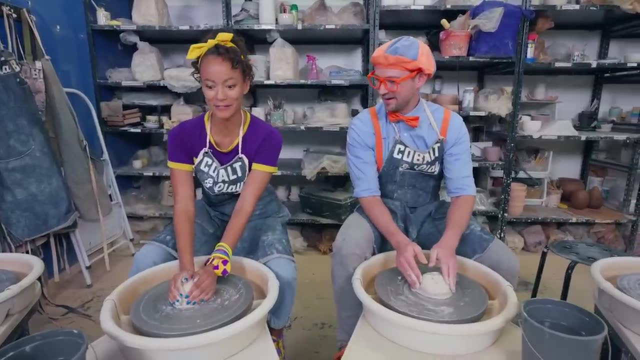 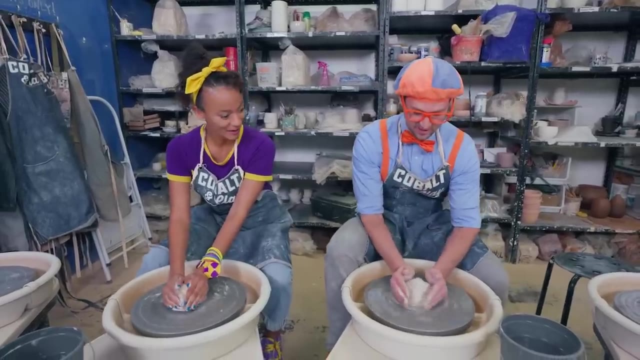 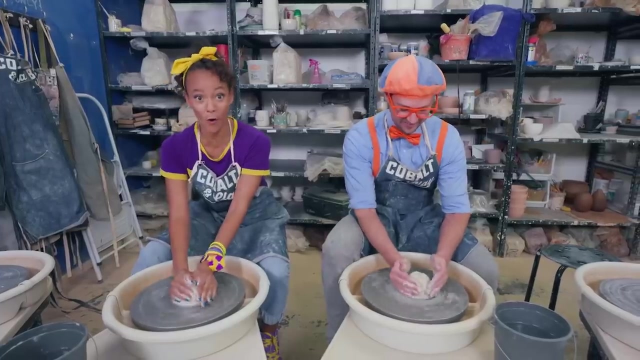 so then it seals from this plate. that sounds right to me. yeah, yeah, okay, okay. well, that's fun really. yeah, wait to try. whoa, okay. oh, it actually goes pretty fast, does it? whoa? yeah, michael is going for a ride. yeah, mine's a little off center so i'm gonna push it in the center. yeah, 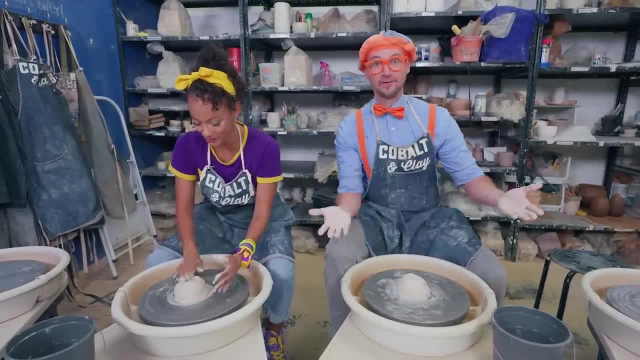 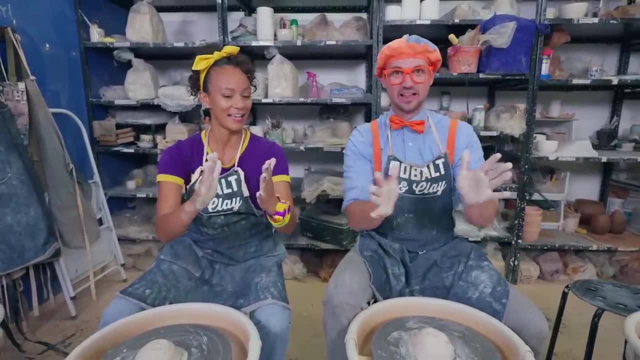 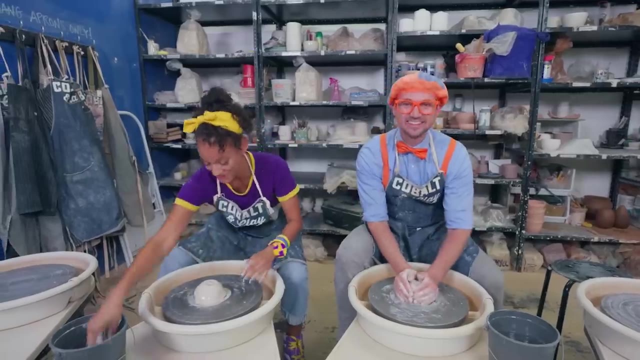 like that. oh, that's a good idea. yeah, maybe it'll work. i don't know whoa. look at my hands. oh, mine too. oh, sticky and slimy. how about a clay high five? oh, stop my face silly doing clay can be pretty dirty, i know, but it's really fun. 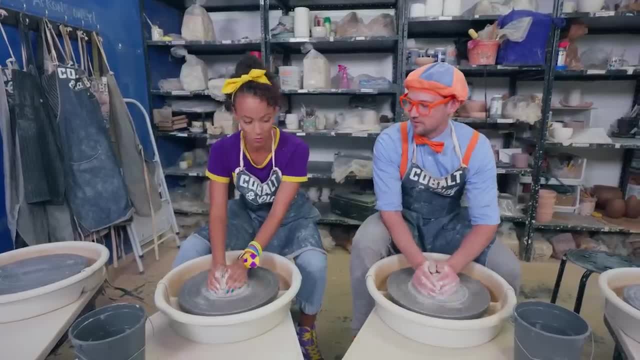 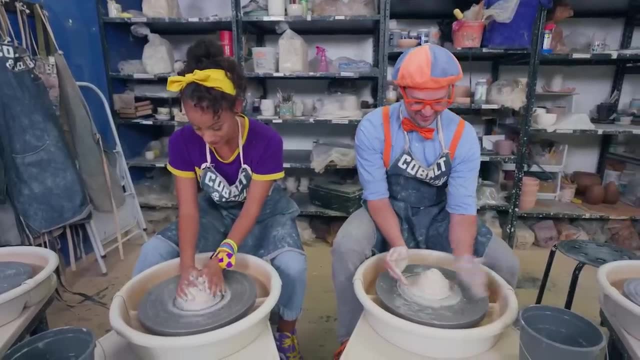 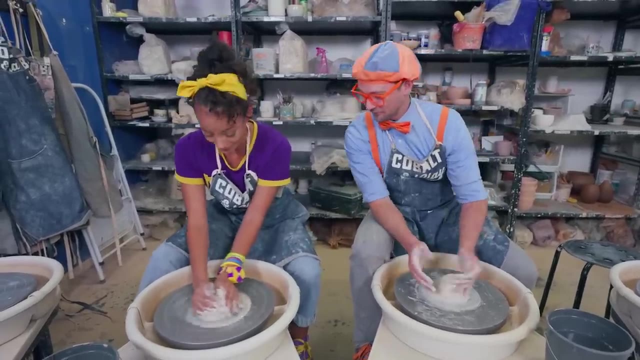 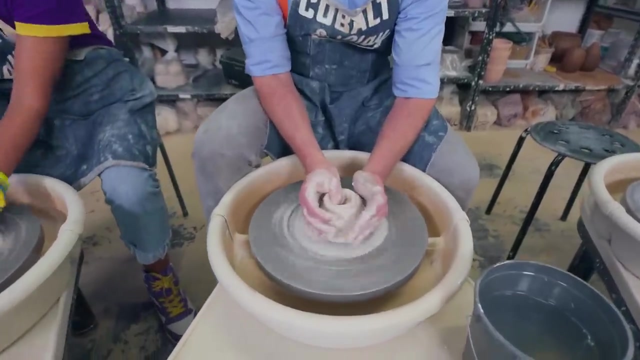 geez, okay, here we go. whoa, whoa, whoa, whoa. okay, don't let go of your clay kid. you're so silly, mika. oh, how are you doing? i don't know, i don't know, i can't stop. it's pretty wobbly. okay, here we go. whoa, look at that. yeah, making a cereal bowl. oh, cool, all right, here we go. 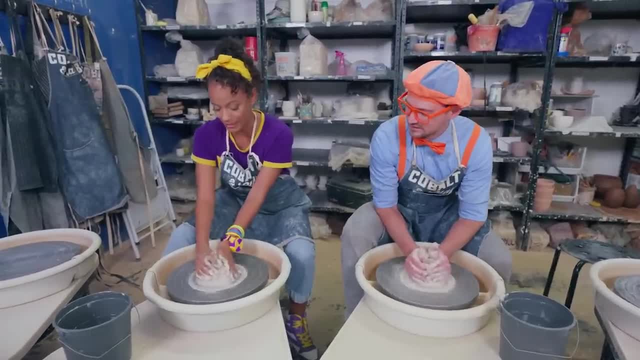 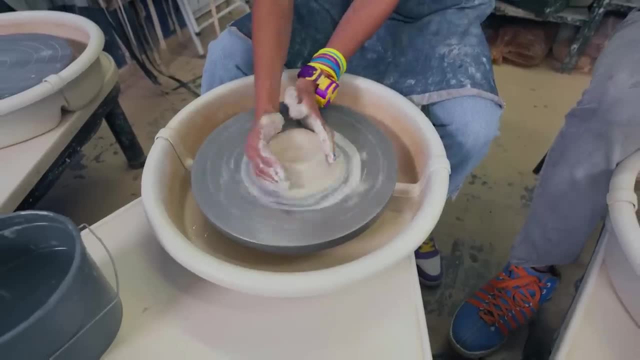 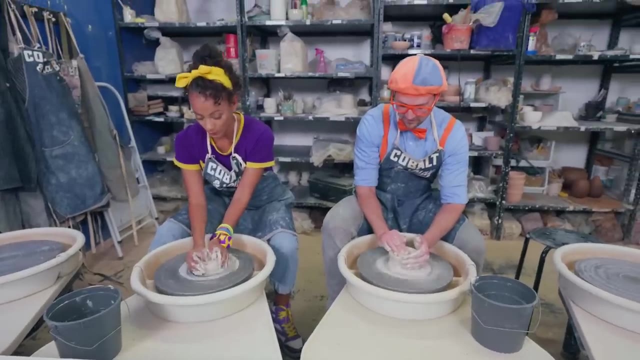 whoa, whoa, i think mine's gonna be a little wobbly. whoa, oh, should we take a look? yeah, let's check it out. oh, okay, i'm gonna keep going with that shape. let's see. whoa, look at what i made. oh, that looks. 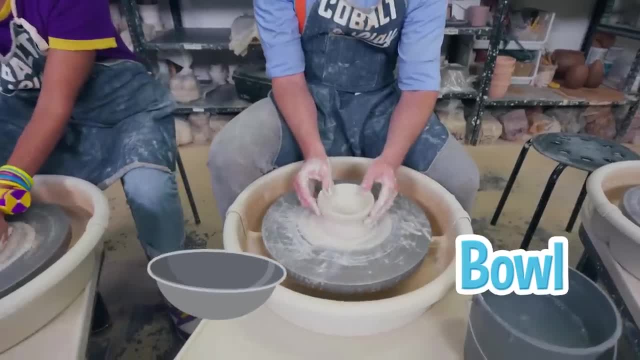 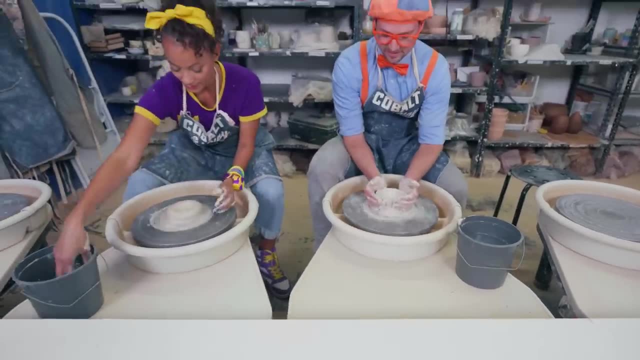 amazing. yeah, it's like a bowl. you can put all sorts of knickknacks in here. yeah, you can put little snacks in there. oh yeah, smart, oh, and it's so cool because when you want to go higher, you just pull it up, you don't. 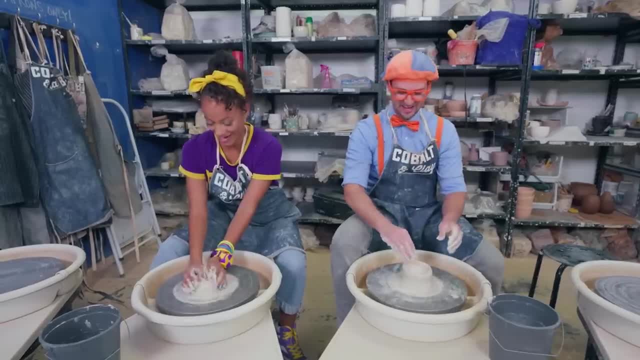 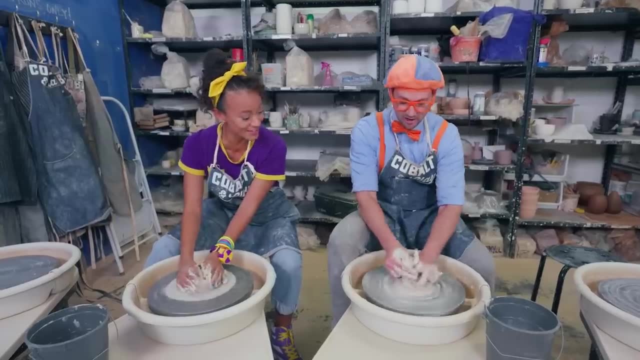 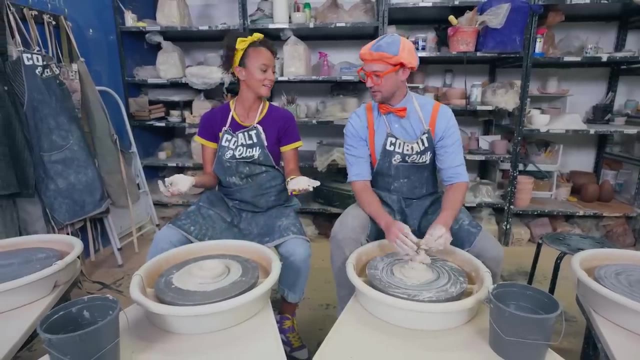 even have to spin your hand around. you're such a natural. thanks, mika, ready, here we go. oh, it's actually harder than it looks. huh, yeah, i ain't broke. oh, yours looks pretty cute, though what, thank you. oh well, shall we go to the nextying box? 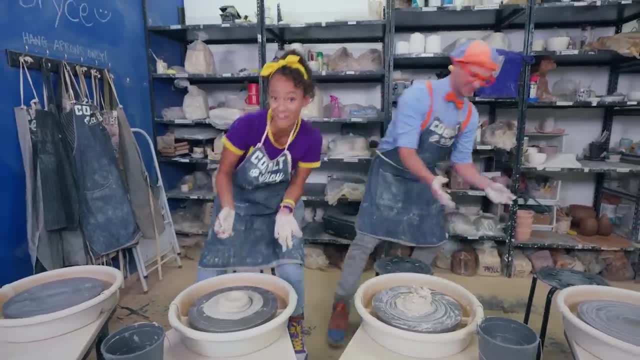 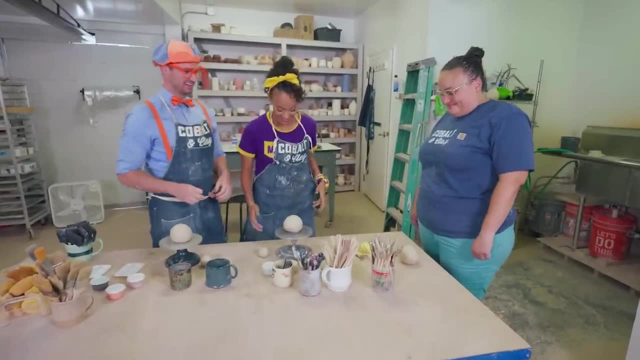 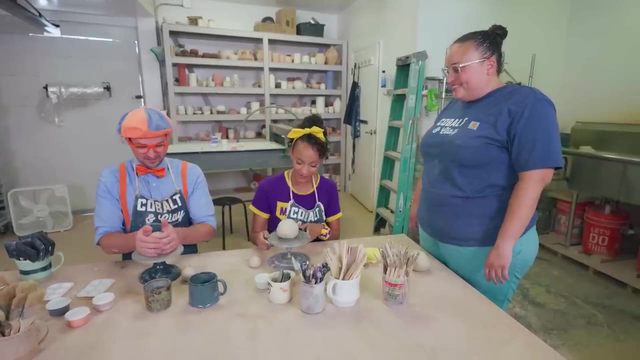 station? yeah, let's try it out. oh, this is fun, all right, come on. okay, washed hands, i think we're ready. yeah, i'm so excited. yeah, all right. and what's this station called? hand building? hand building- whoa, so do we build with our hands? yeah, we're gonna um sculpt our animals right now. oh, 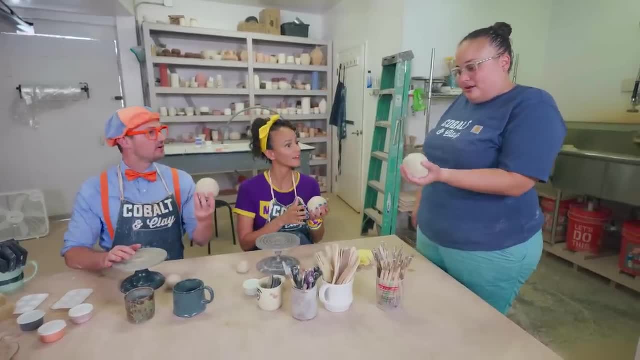 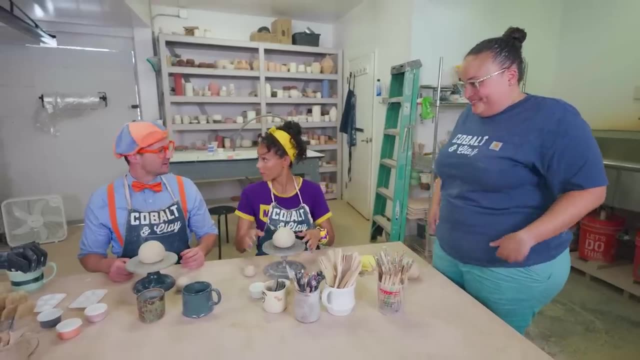 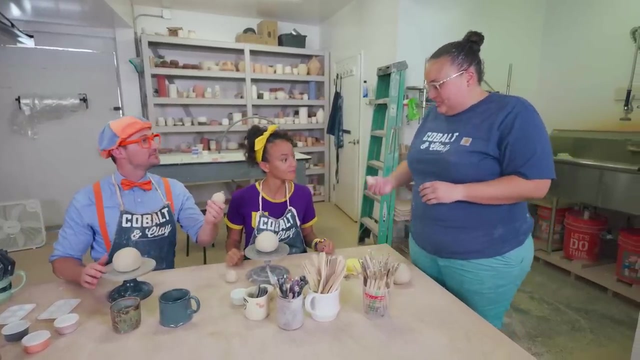 okay, is this the body or the head? this is gonna be our animal body. oh, okay, fun. look at this. wow, it's kind of like the wheel we were out before, but smaller. it's okay. and what's this one for? we're gonna use these to make our attachments so like the. 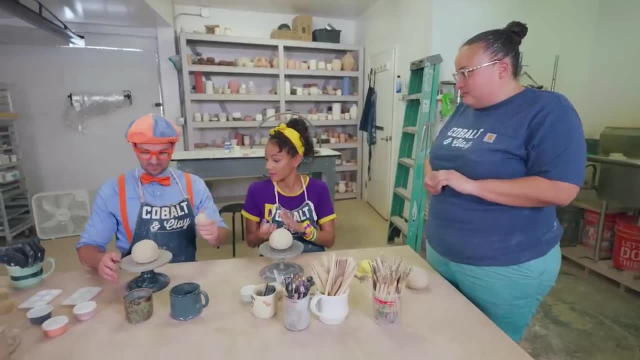 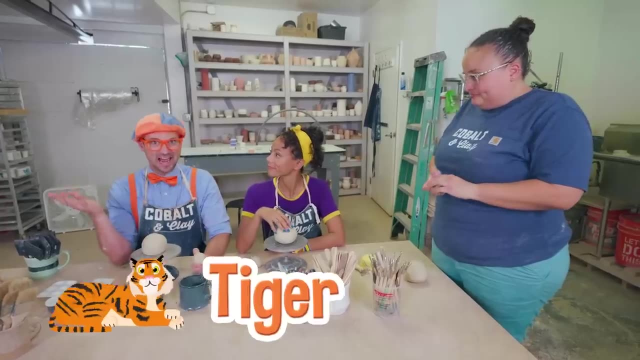 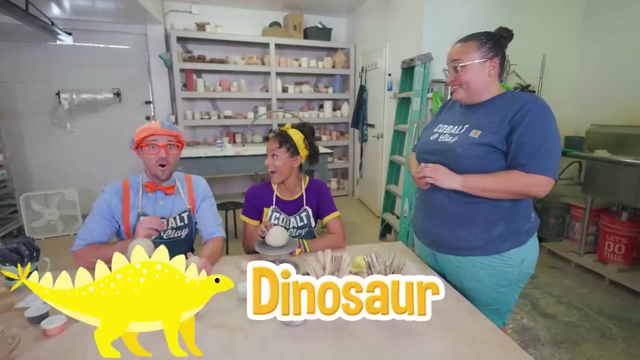 animal's limbs and maybe like some fins or some, whatever you're trying to create. oh cool. well, huh, what kind of animal do i want to make? um, maybe a tiger? oh, that's a good one. yeah, what about you? i think i might do a dinosaur, oh fun. 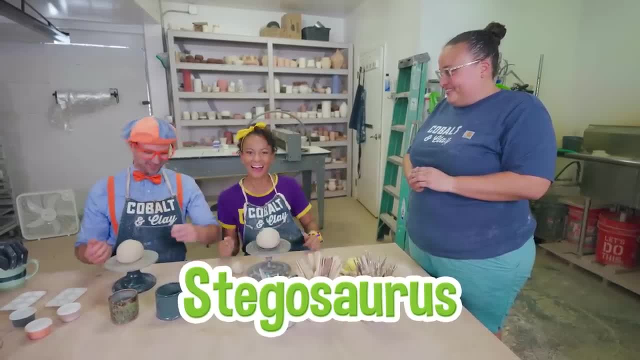 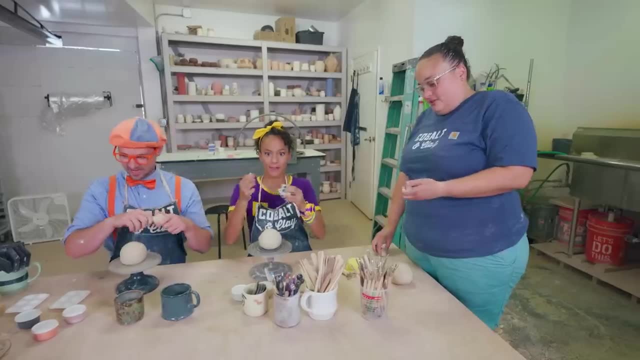 plates down the back. oh, like a stegosaurus. yeah, cool, all right. so how do we get started? just pull it off, yeah, so you're going to just pinch a little piece of clay off, okay, and then you're going to roll it. use your fingertips to mold the shape that you'd like. so if you're trying to make 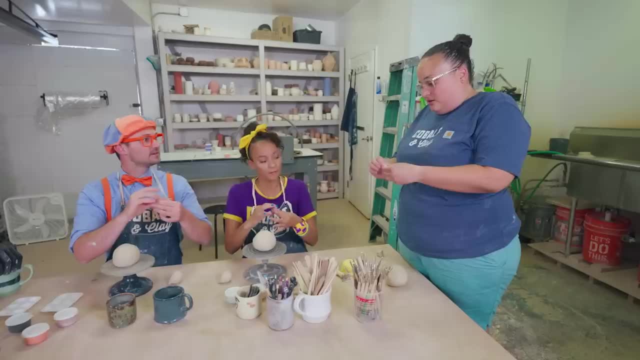 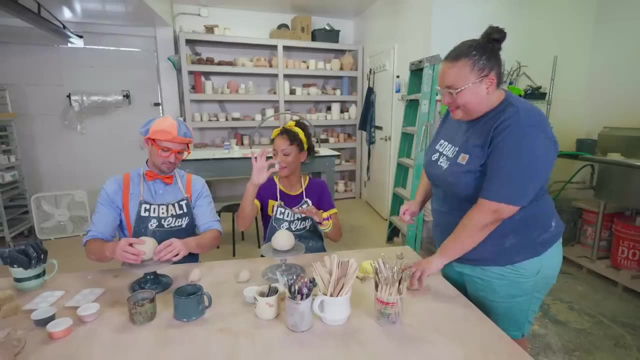 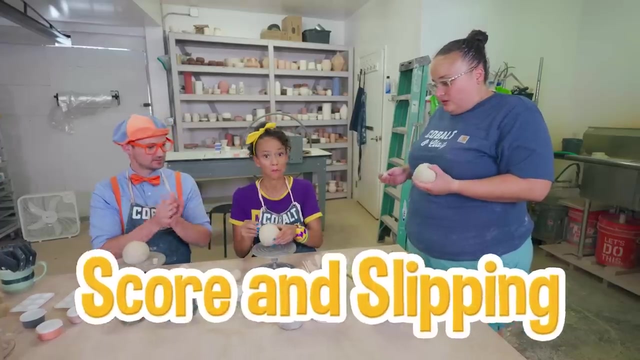 um, if you're trying to make a limb, then you know you just want a little foot or a paw of some sort, right? yeah, look at this, a really short leg. yeah, nice, okay, and how do you get it to stick out? so when you make clay attachments, it's called score and slipping. so what we need first is needle. 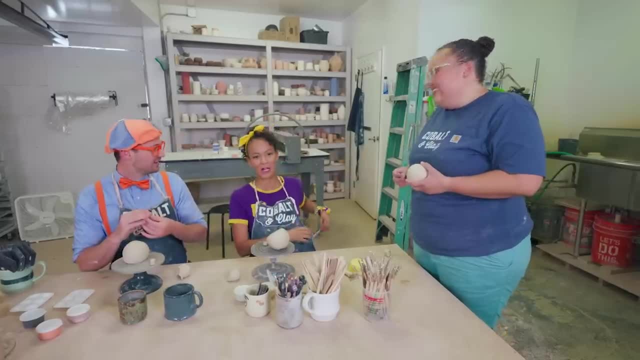 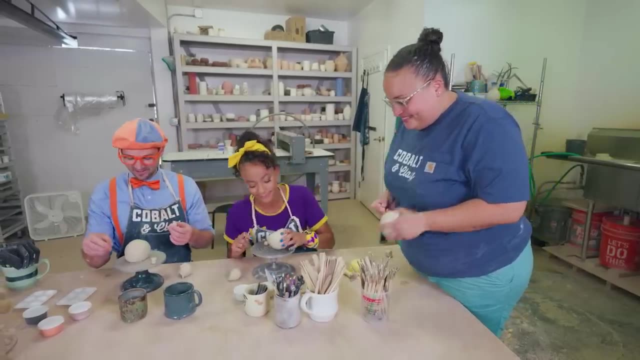 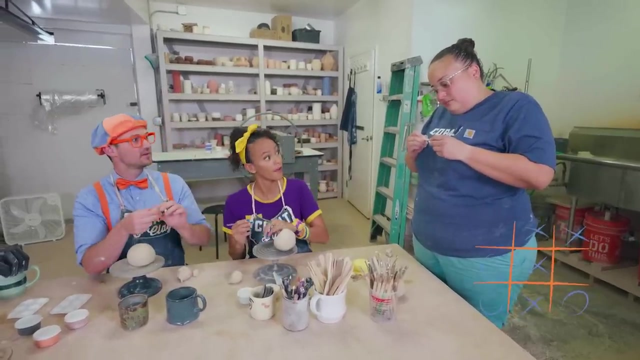 tools, needle tools. you could just have these needle tools in your jam pack. i mean, you got anything in my jam pack, oh cool, okay. so how do you do it? so, my god, so you're going to take the needle and then we're going to make a little tic tac toe mark on one of the bottoms of our piece. okay, okay. 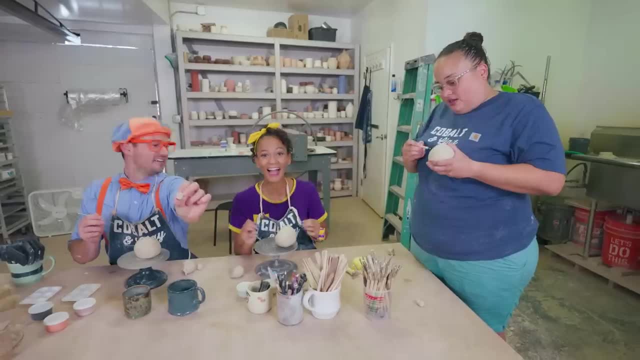 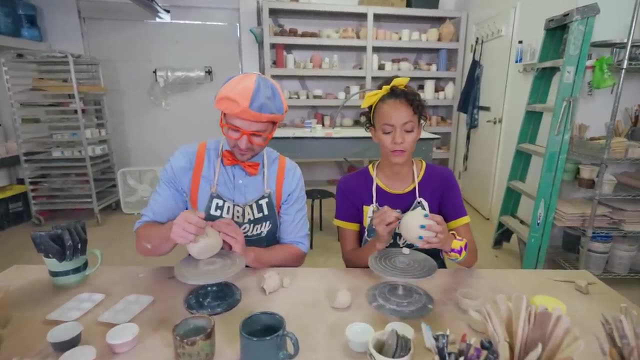 what a fun game. And then you're going to do it to the body as well, where you're going to connect it? Okay, Where should I connect it? Okay, how about? right here? One, two, three, four, Okay. 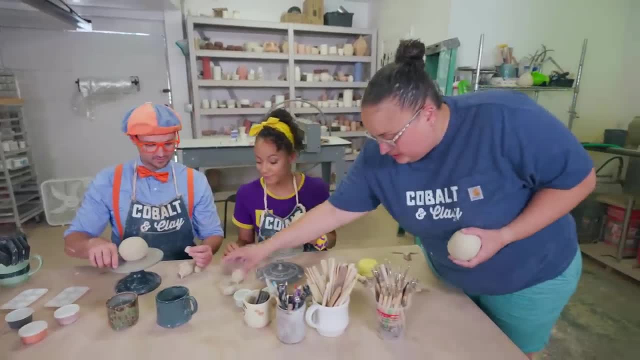 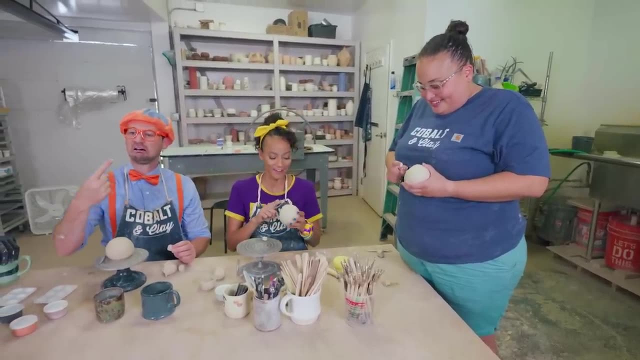 There we go, All right. And then in these cups, these are called slips. So what you're going to do is you'll dip your finger in the slip. Oh, like glue, It's clay glue. basically, You're going to dot the tic-tac-toe. 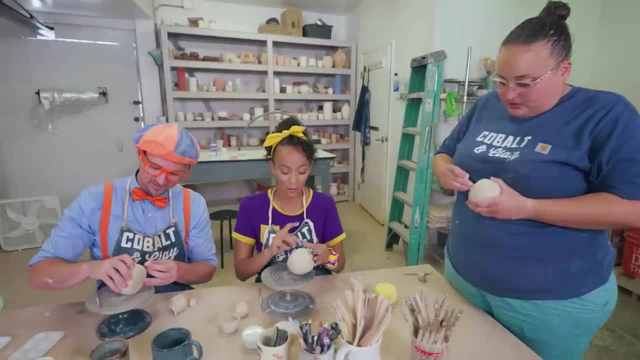 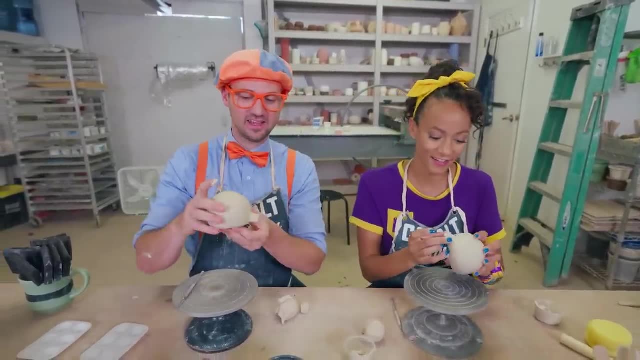 You'll put them together and then you'll firmly push it so it could stick to one another. Okay, There we go Together. Oh yeah, it's sticking. Oh yeah, It did Check it out, Oh cool. 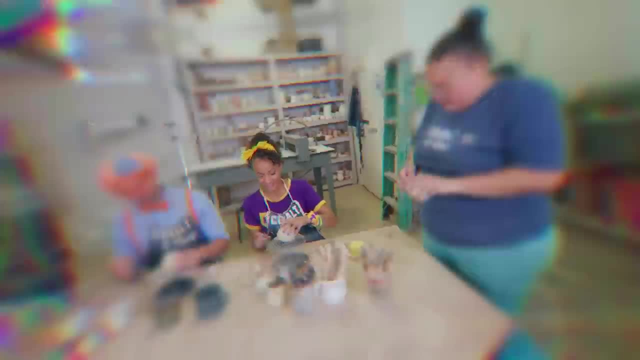 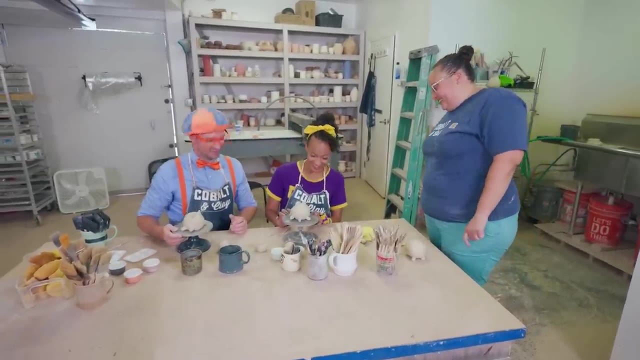 Look at mine. Good job, One leg done. There we go. That looks so good, Blippi. Oh, yours too. Oh, thank you. Wow guys, your animals look great, Thank you, Thank you. What do we do next? 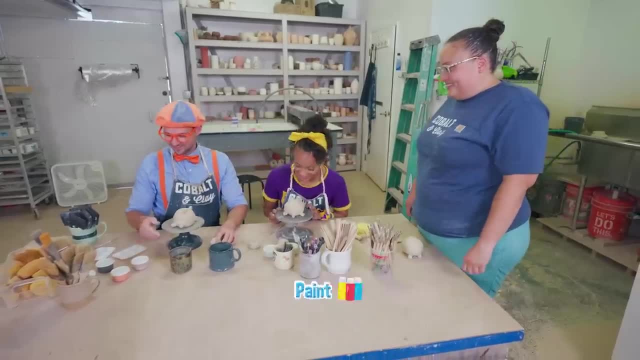 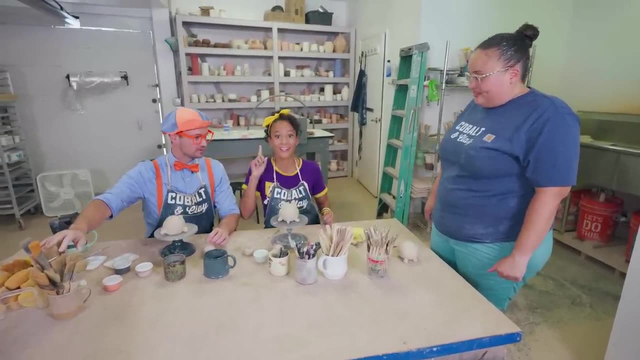 So now we're going to paint them. bring them to life, Paint them Cool. It looks like we have some paint right here. Oh yeah, But these brushes look way too big. Oh Oh, don't worry, I have paint brushes right here in my jam pack. 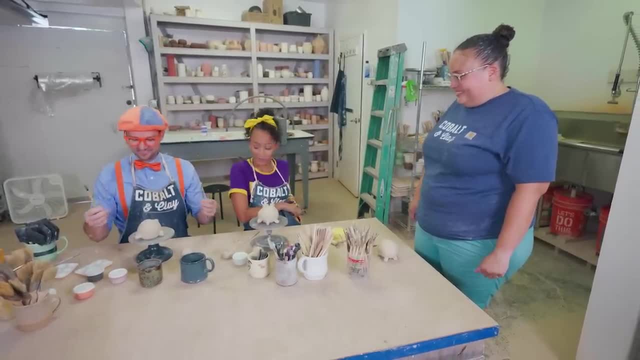 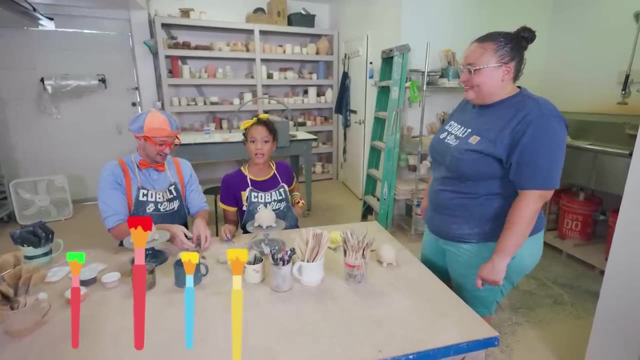 Oh, you have everything in there. I really do. I have some more too. if you want other options, I have a little one, I have a bigger one, I have another little one. I also have a medium-sized one, Whoa. 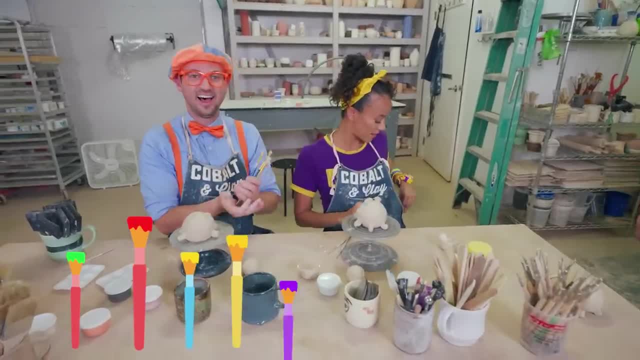 And I also have another one that's: oops, sorry, that's not it, That's a tool, And I have a tiny one and I have another tiny one. Whoa, Okay, I'll use this one and this one. 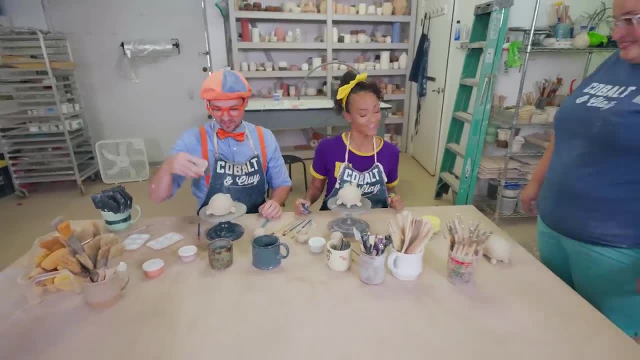 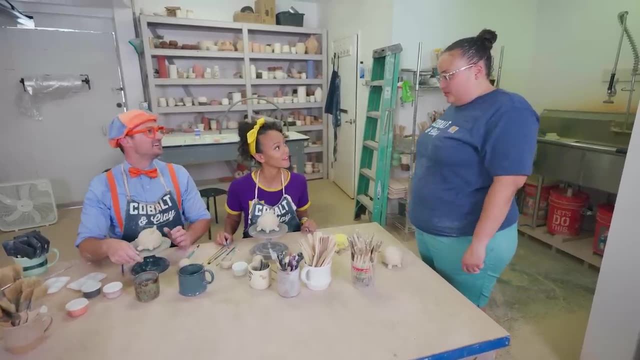 Okay, sounds good. Oh, and then we just use these paints and put them on the animals. Yes, Whatever color you want it, whatever designs you want, you're going to dip it in and then you'll just paint it onto your animal. 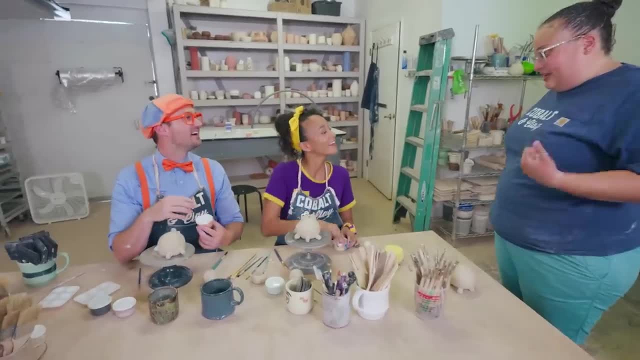 Awesome, Thank you, Let's do it. Yeah, since you guys have what you need, I'm going to go check on the kiln and I'll come back and I'll have a check on you. Okay, thank you Thanks. 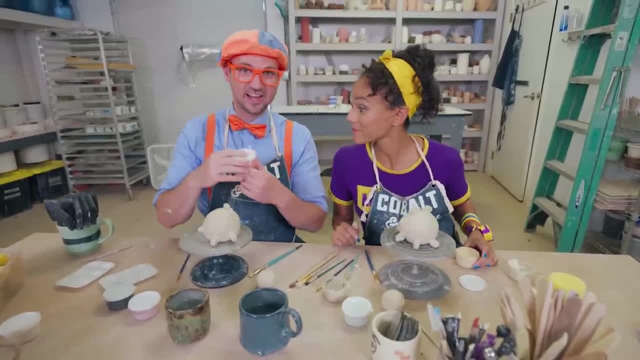 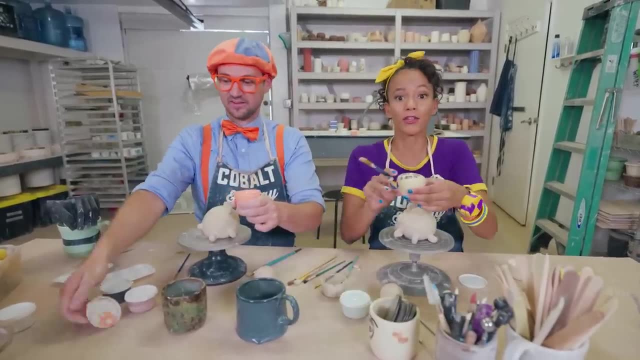 See you, Whoa, cool. Okay, since I'm doing a tiger, I'm going to use orange. Oh, good idea, Whoa, And I'm going to use yellow for my dinosaur. It doesn't look like yellow right now, but once it's baked, it's going to turn to a nice. 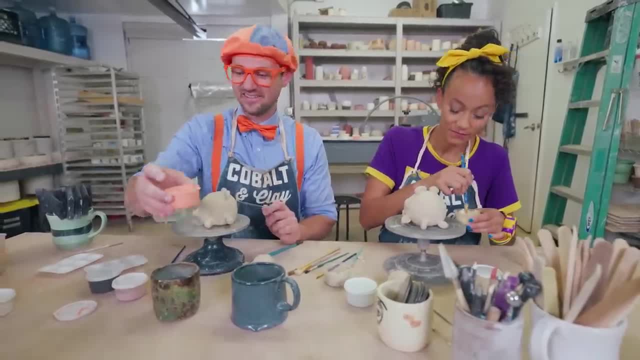 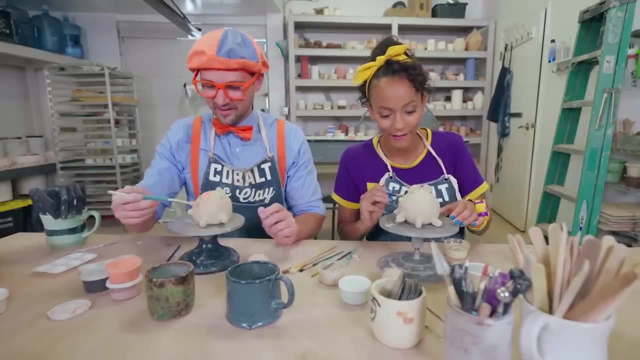 bright yellow. Oh, cool, Cool, Check this out. Ooh, Ooh, There we go. Okay, Okay, Here we go. I've never painted clay before Me, neither. Whoa, it's really fun, Oh see. 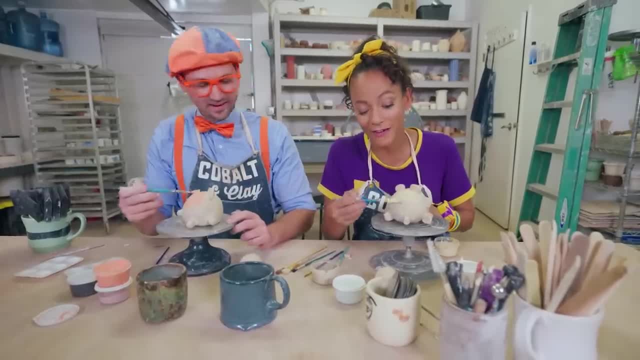 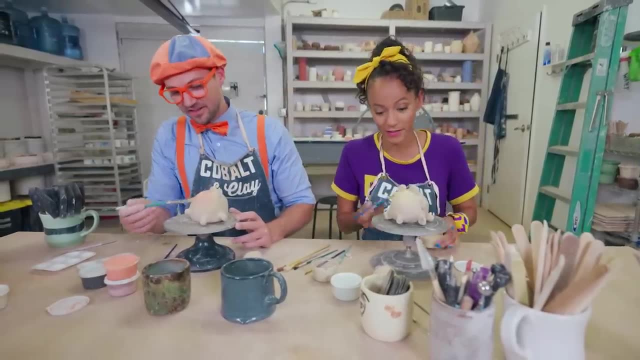 Whoa. Right now it looks like the same color as the clay. I can't wait to see it when it's yellow. Yeah, My orange isn't that bright, but I bet after it gets fired in the kiln then from there. 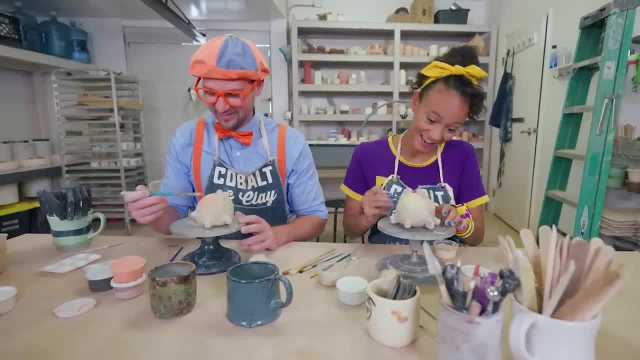 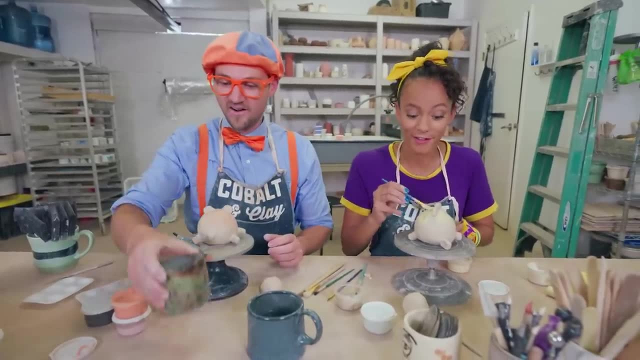 I bet it'll turn really bright orange. Oh yeah, Oh, Oh look Water Pretty thirsty. No, no, Blippi, What That's for your paintbrush. Oh, Smart Yeah, You dip your paintbrush in this water. 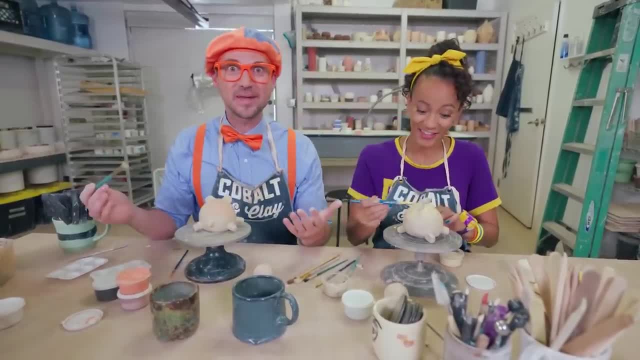 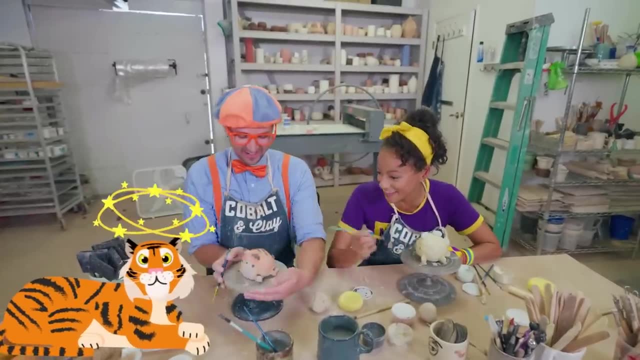 You don't drink it, And so then you can use a different color without mixing them. There you go. Oh, thank you, I got you. I'll get some water later. Whoa Dizzy tiger. Yeah, Look at that. 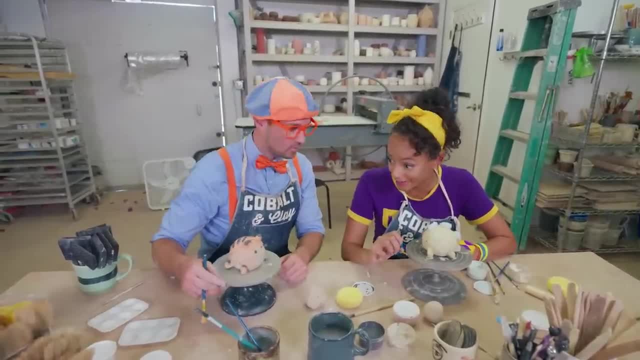 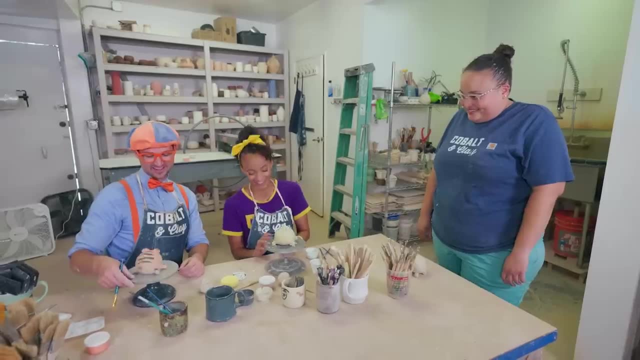 Whoa, This thing's so cool. Yeah, Hey, your tiger looks really good. Wow, Yours too. It's so colorful. Thank you, Oh, hey, They look great. Thank you, Yeah, You like them, They're amazing. 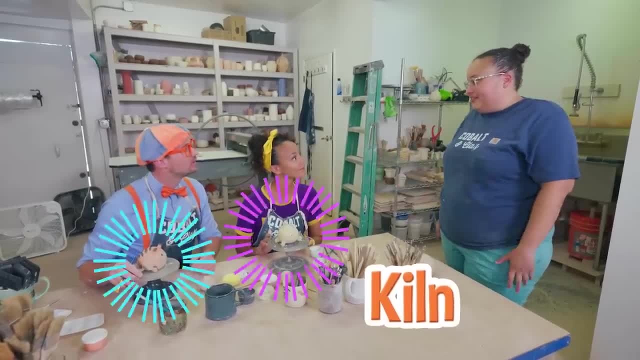 Whoa, Why aren't they so bright and colorful? So once we take them and put them in the kiln, the colors are going to get a lot brighter. Oh cool, Can't wait to see them. Yeah, So is my orange going to get, like my suspenders and bow tie. 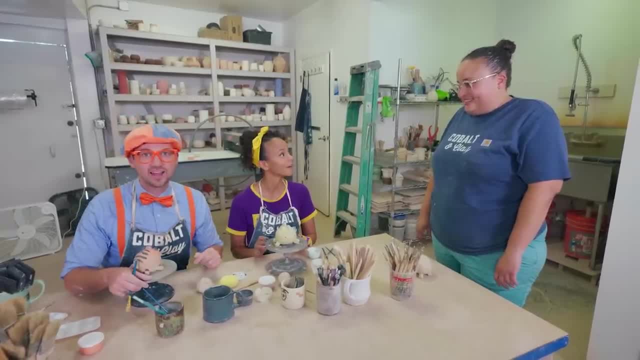 Exactly Whoa. And will mine get as bright of a yellow as my headband? Yes, Oh, that's fun. Whoa, Oh cool. Well, what do we do next? Well, what I'm going to do is I'm going to take your guys' animals, and then I'll put. 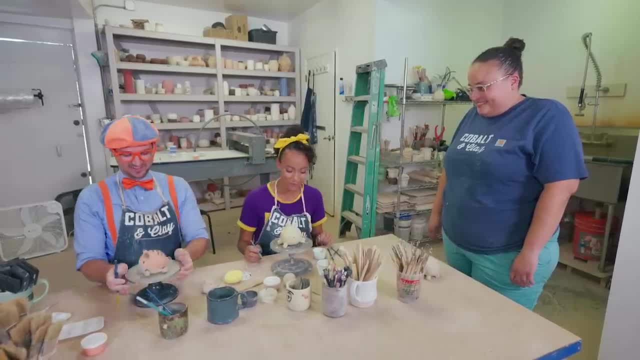 them in the kiln, and then I'm going to put them in the kiln, and then I'm going to put them in the kiln, And then you can come get them when they're ready. Oh fun, Sounds like a good plan. 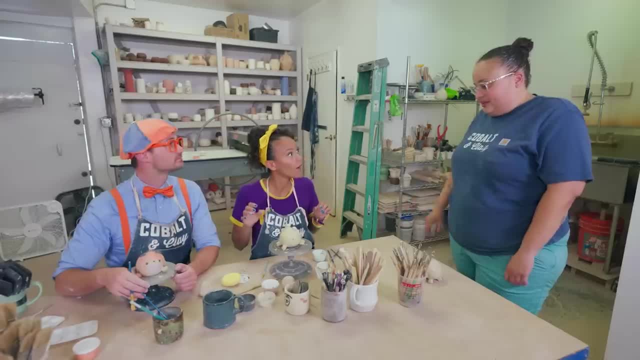 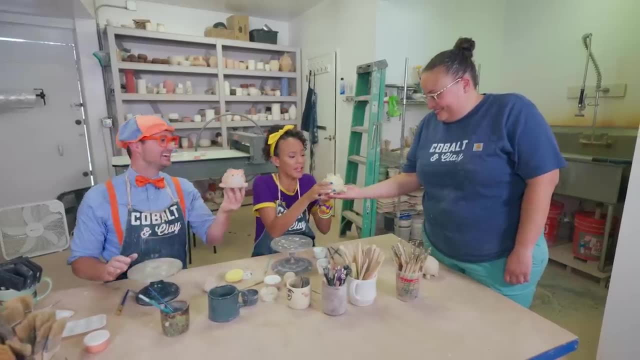 Okay, Here you go. See you later, Tiger. Okay, Be gentle with it, Here you go, Thank you, Bye. Well, thank you so much. Aw, See you. Wow, That was so nice for teaching us about pottery. 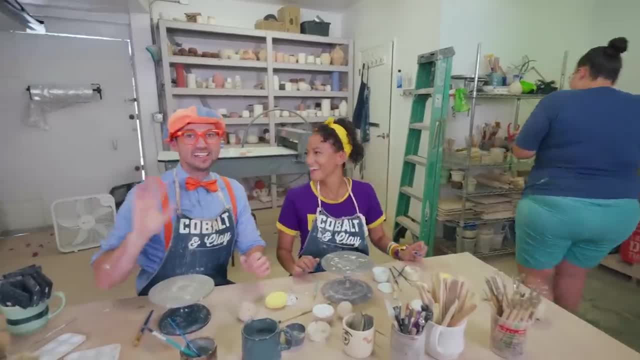 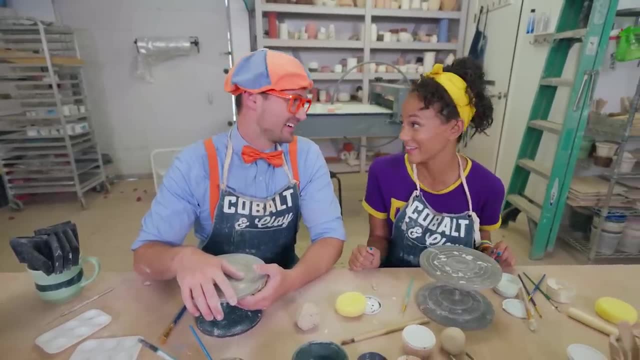 Yeah, That was really nice. We learned a lot. Yeah, Can't wait to see what they look like. I know That was really fun. Yeah Well, thank you so much. Bye, Bye, Bye, Bye, Bye. 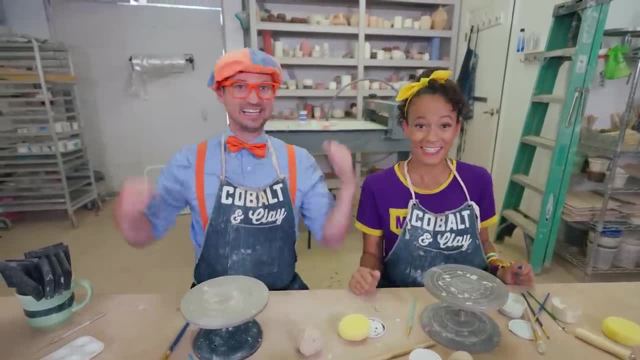 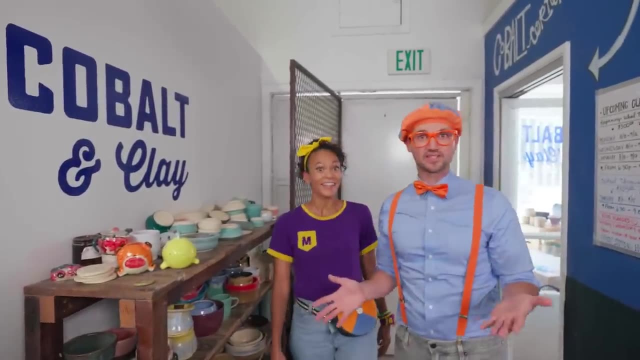 Well, shall we return the aprons? Yeah, Let's do it, And then we can come back to pick up our things. Great idea, All right, Woo-hoo, Whoa, Look at these, Look Cool. This must be where everyone picks up their pottery. 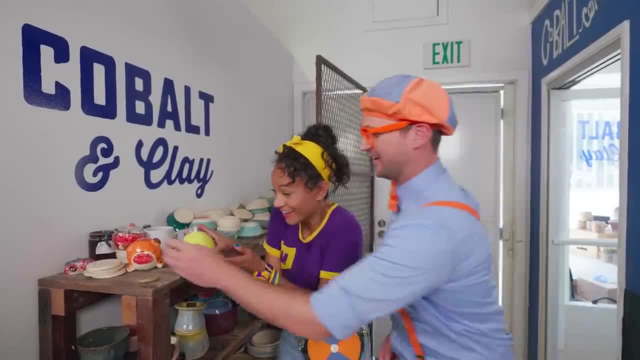 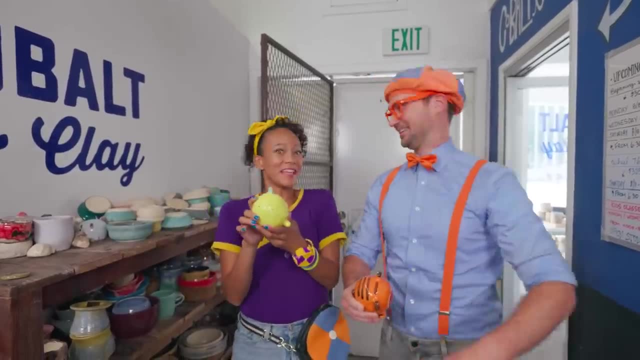 Yeah, Ours, Yeah, Cool, What do you think? Oh, She's right, It did turn bright orange. Yeah, It really did, And mine turned bright yellow. Oh, Yours look so great. Thank you, I really like yours too. 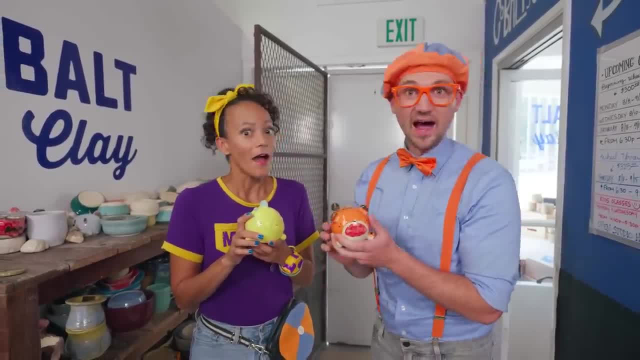 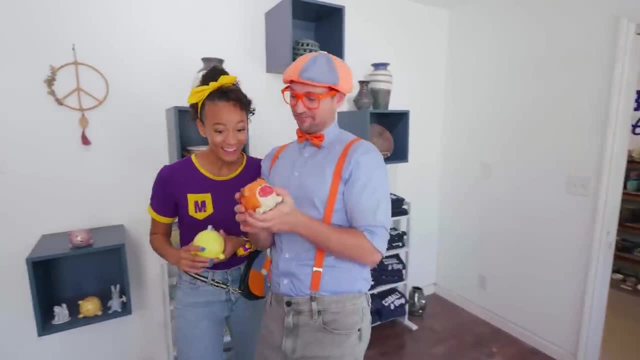 Aw, Thanks, Shouldn't we go? Yeah, Put it by the pig. Yeah, Let's go, Come on. Uh-oh, That was so much fun today. Yeah, That was a great time making these new friends, Yeah. 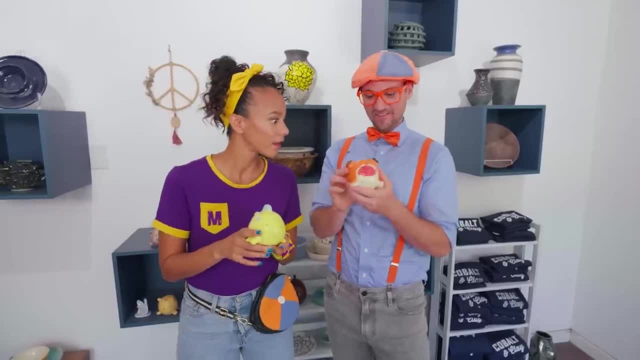 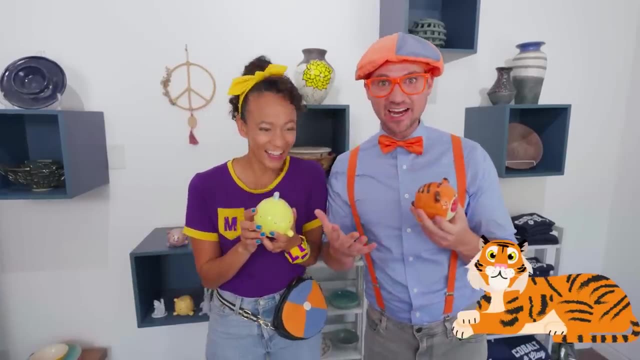 Whoa, Hey, Did you notice They both roar. That's right, Because mine's a dinosaur And mine is a tiger. That's cool. Should we roar together? Yeah, Will you roar with us? Ready Roar. 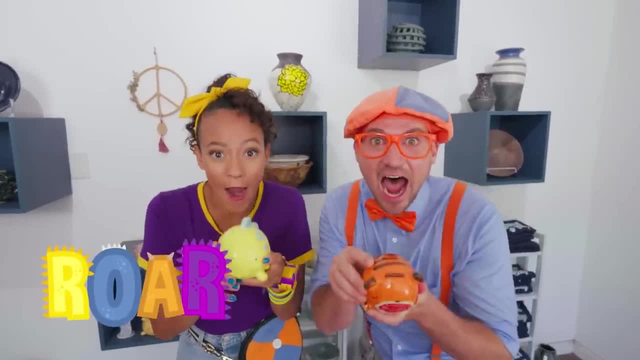 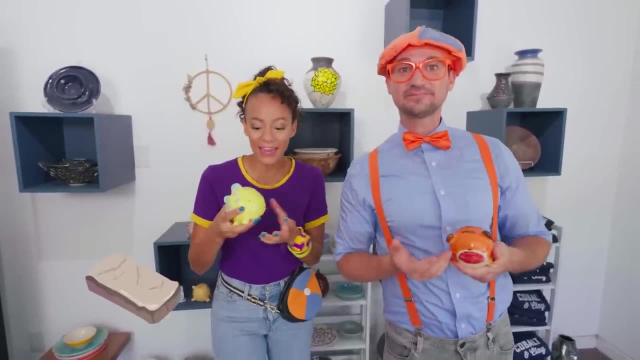 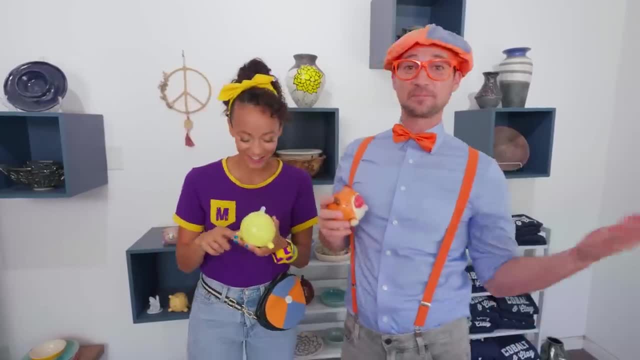 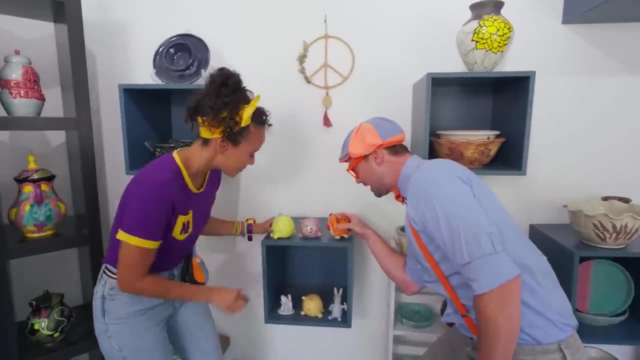 Yeah, Oh, Making art is so fun, Yeah, Especially with friends. Yeah, Oh, Speaking of friends, Oh yeah, Hello, Will you be our friend? Please say yes, Please say yes, Yes, Yeah, We did it. 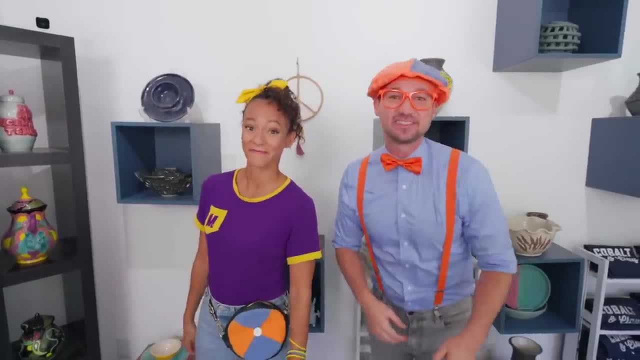 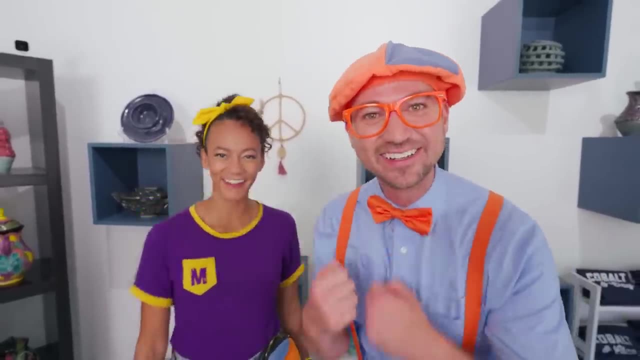 Nice job, Good job. Well, this is the end of this video, But if you want to watch more of my videos, all you have to do is search for my name. Will you spell my name with us? Cool B-L-I-P-P-I.